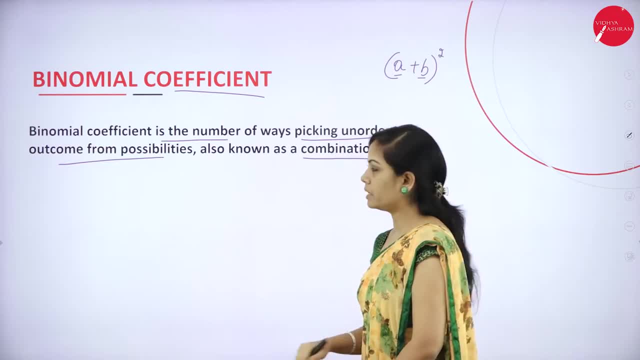 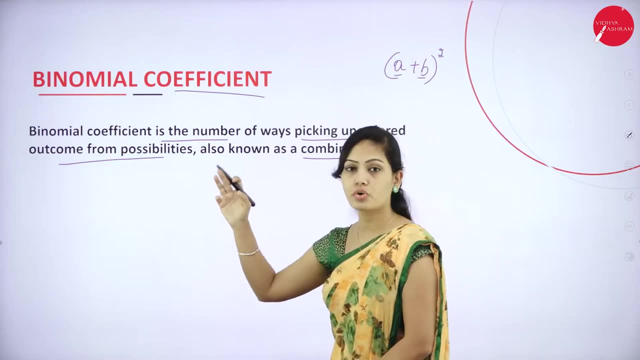 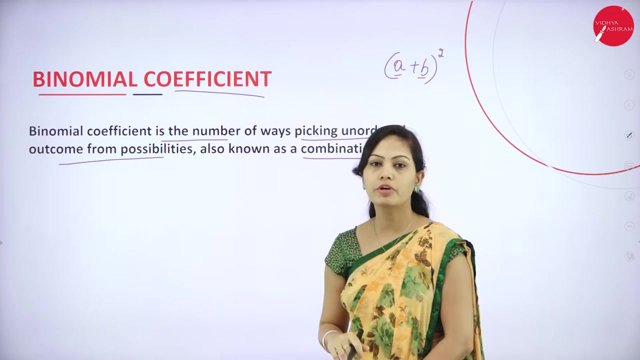 picking the unordered outcome from possibilities, also known as a combination Clear. So here an expression contains two terms are known as binomial. Binomial coefficient is the number of ways picking a unordered outcome from possibilities. So here an expression contains two terms are known as binomial. 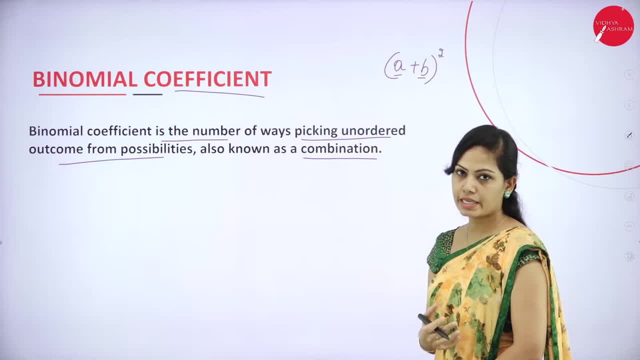 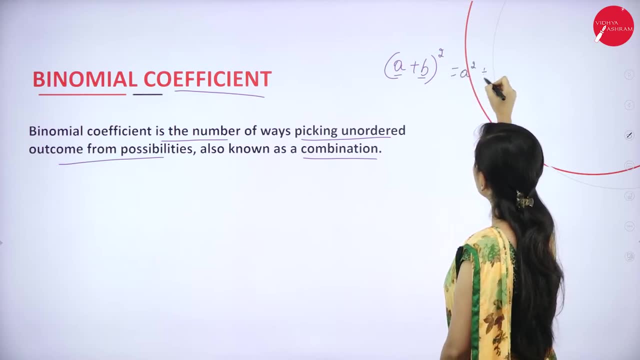 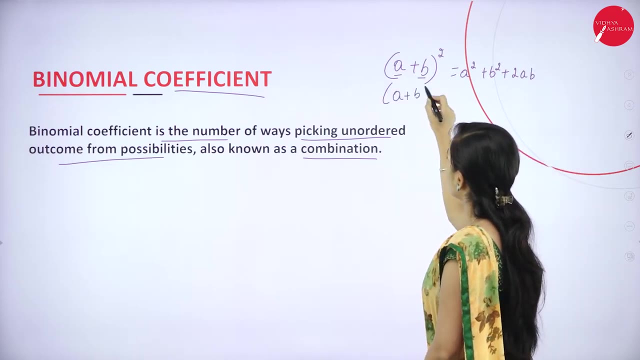 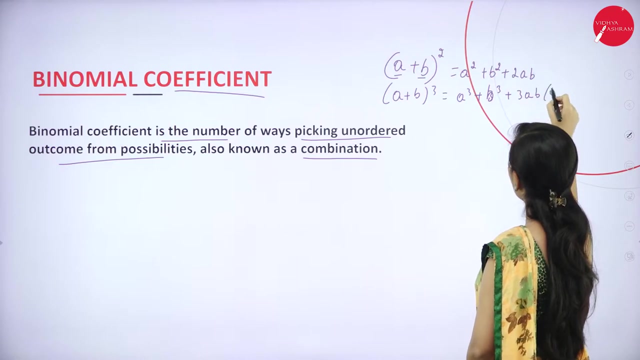 possibilities. and what is this binomial expansion? so we have a plus b whole square. so a plus b whole square means it is a square plus b, square plus 2ab, right? so what is a plus b whole cube? a plus b whole cube is equal to a cube plus b, cube plus 3ab into a plus b. so again you can simplify this. 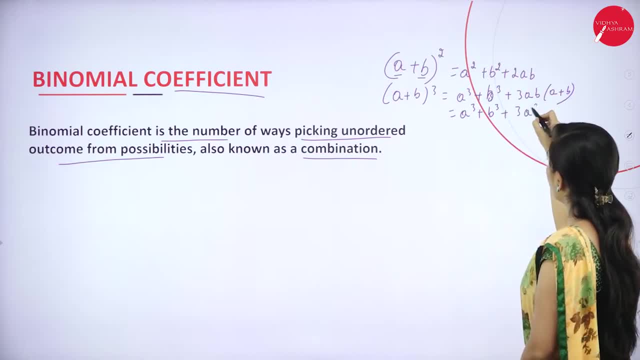 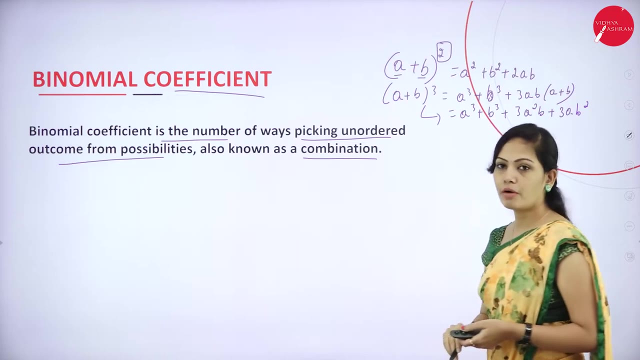 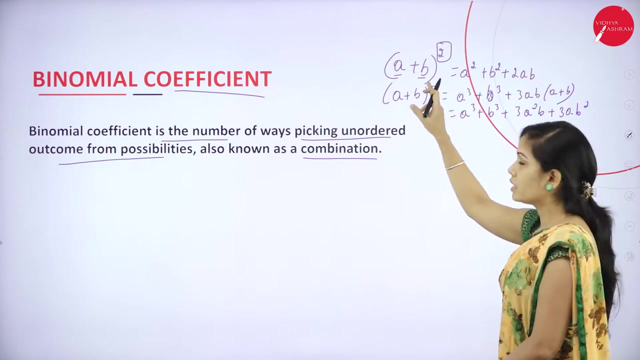 a cube plus b cube plus 3a square, b plus 3ab square. so a plus b whole cube means a cube plus b cube plus 3a square, b plus 3ab square. so if you get power 2, so you will get 3 terms. keep in mind: if your power value is 2, then you will get 3 terms, right. if your power value is. 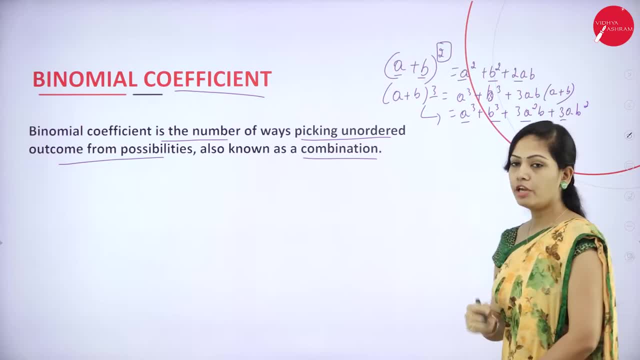 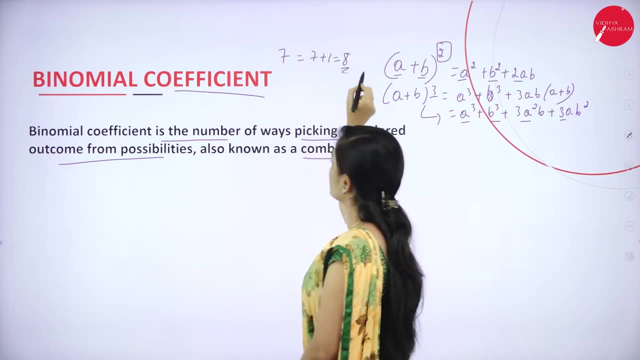 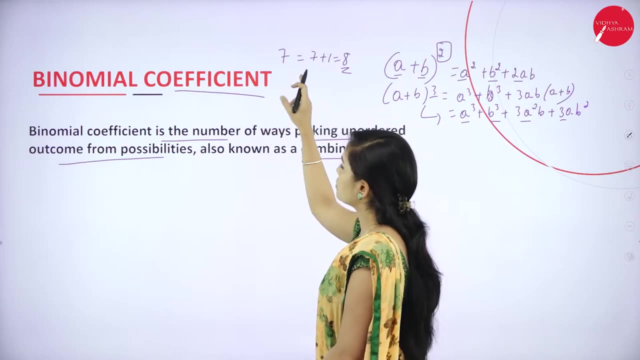 3, 3 will get 4 terms. If your power value is 7, you will get 7 plus 1 is equal to 8 terms In binomial expression or binomial coefficient in the expansion of binomial. so if you get power value is 7 or 6, 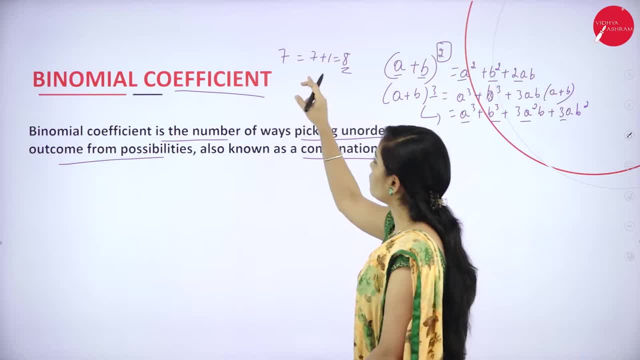 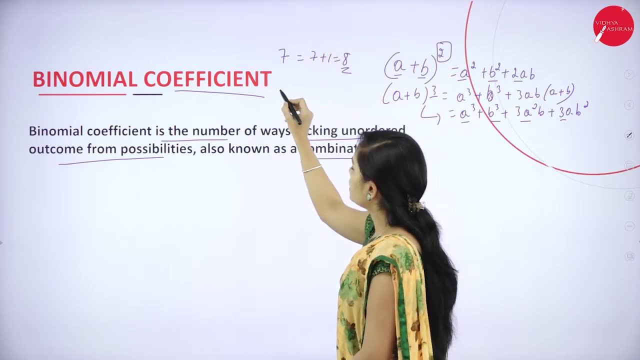 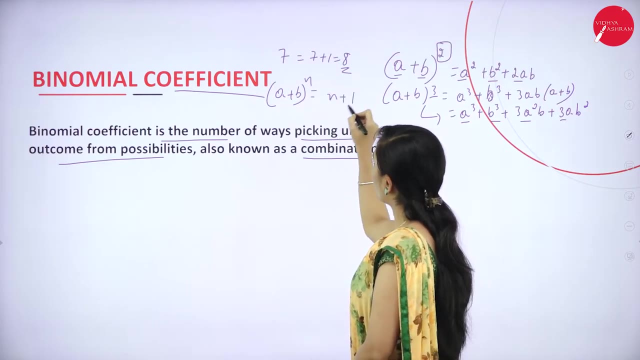 or anything in binomial expression, the power value is 3, you will get 3 plus 1 times, So in 3 plus 1 terms. example, if your power value is a plus b, power n, so you will get n plus 1 terms clear and 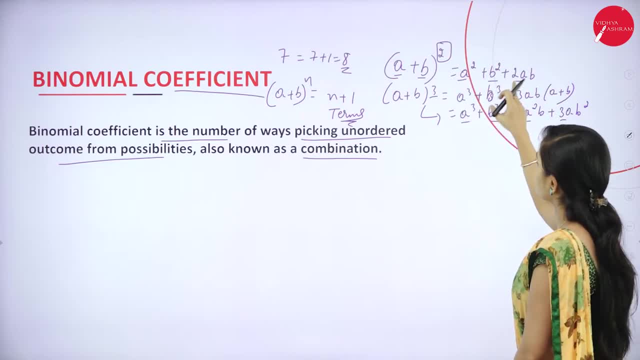 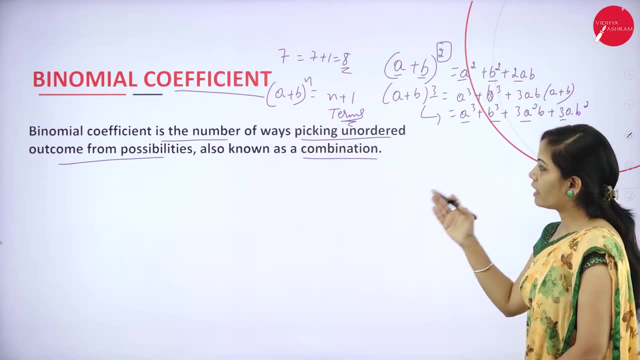 here a plus b whole square is equal to a square plus b square plus 2ab. we have 3 terms here. we have 4 terms, clear. So if your power value is n, you will get n plus 1 terms. Now see the expression. 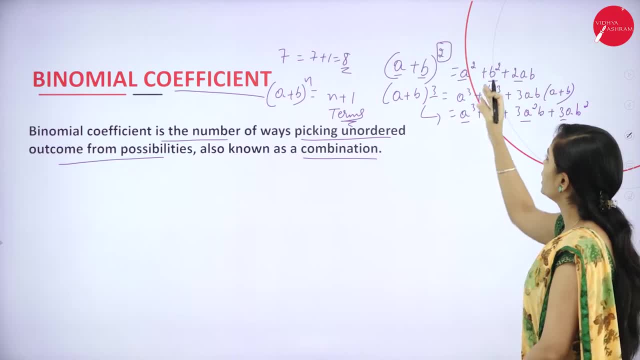 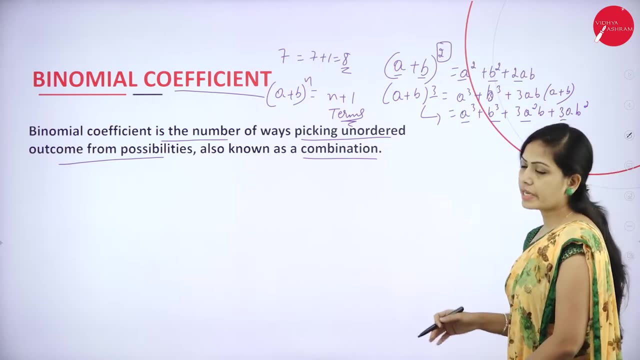 a plus b power square power value is 2.. So easily you can apply a plus b whole square formula, so you will get this expression right. If your power value is 3, you can apply a plus b whole cube formula and your expression is 2x plus. 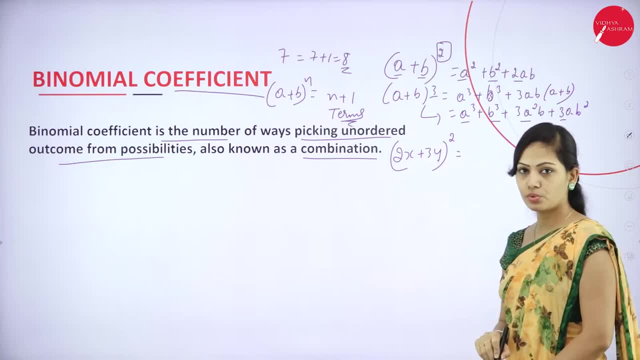 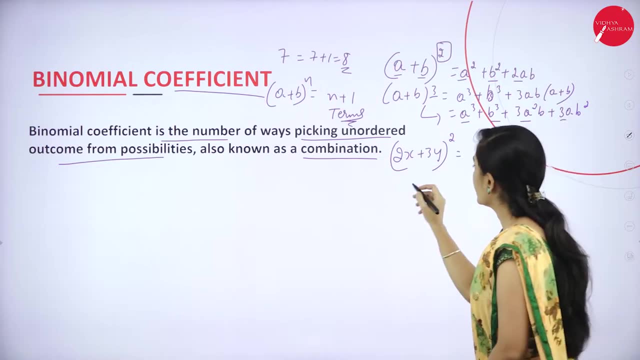 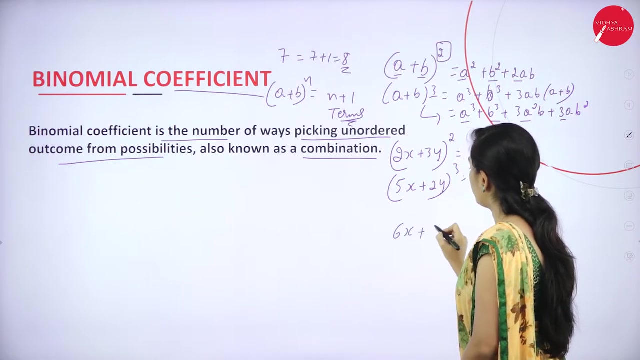 3y power value is 2.. So you, easily you can apply this: a plus b, whole square formula right. You can simplify this easily. and if you get 5x plus 2y power 3, you can apply This a plus b, whole cube formula right. and suppose: if you get 6x plus y, whole power 5. if you are 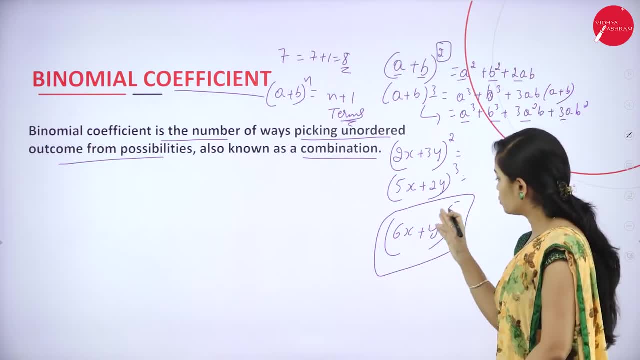 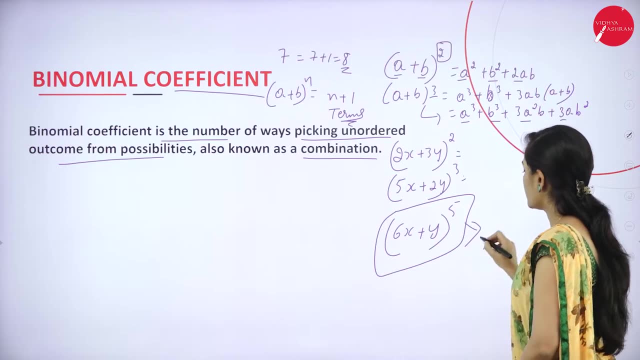 applying a plus b whole square formula, a plus b whole cube formula to this expression. it will be very difficult because power value is 5, right? So for that we are using this binomial expansion clear. by the help of binomial expression we can simplify this: 6x plus 2y, power 5.. So you can simplify. 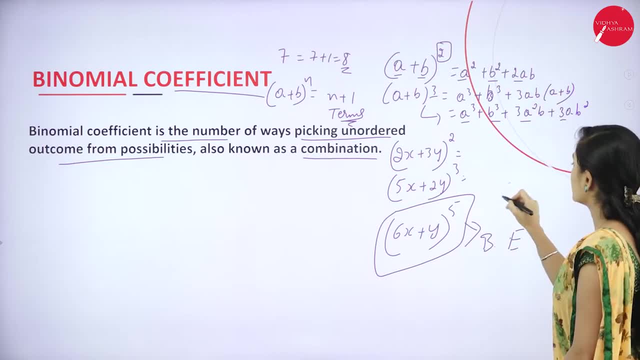 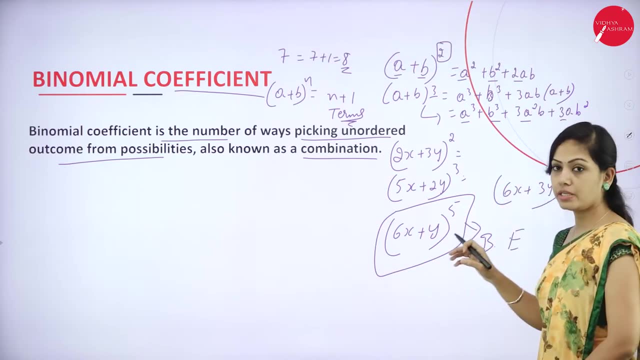 6x plus y power 5 or 6x plus 3y power 12.. You can simplify this power value right So easily. you can simplify any power value using binomial expansion and you can also simplify this 7x plus 3y power. 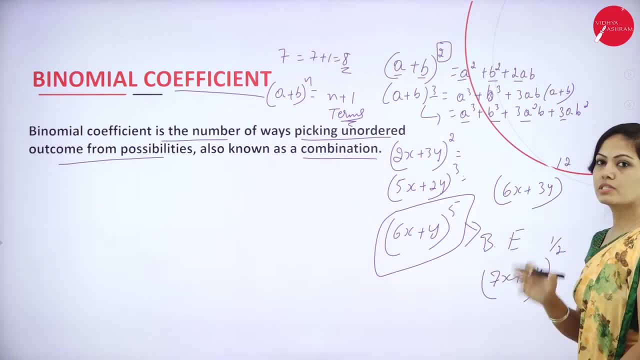 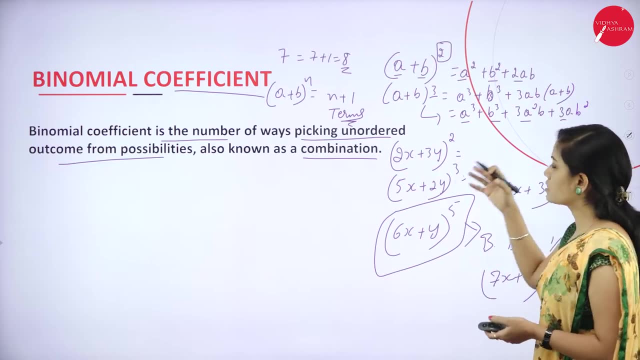 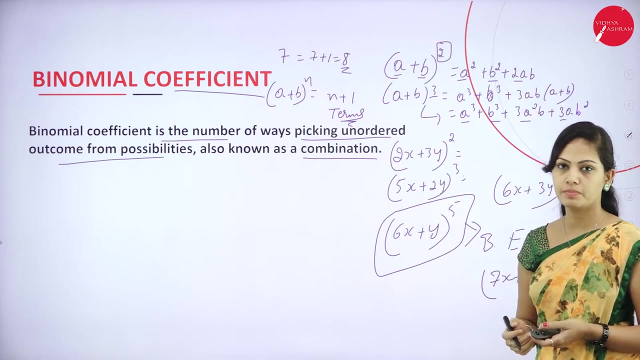 1 by 2 clear This power. also, you can simplify using this binomial expansion Coefficient concept. If your power value is more than 2 or more than 3, so easily you can apply this binomial coefficient concept. So what is the binomial expansion formula? So example x plus a: 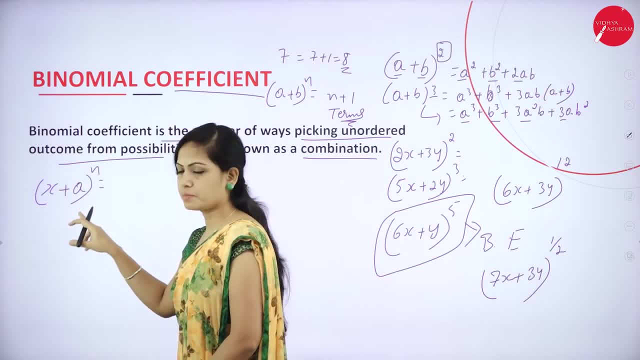 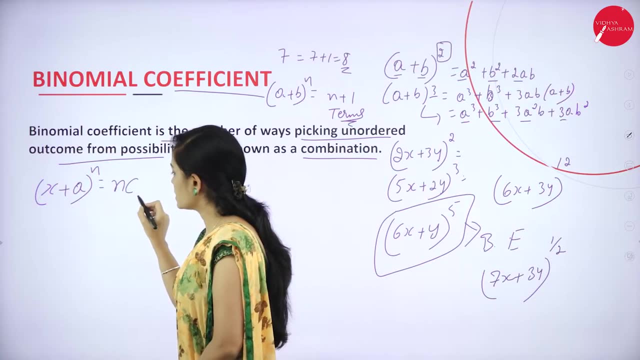 power n. Here I have an expression x plus a power n, So now I will use combination nc 0- nc 0.. So I have an expression nc 0- nc 0.. So I have an expression nc 0- nc 0.. So I have an expression nc 0- nc 0.. 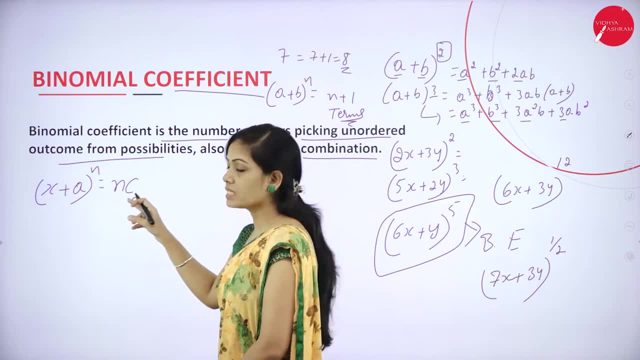 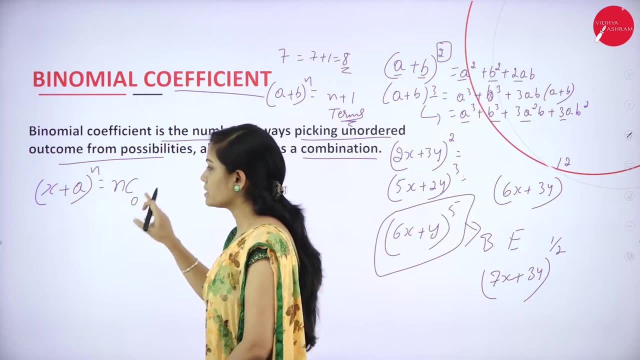 So I am using combination ncr formula. So what is ncr? ncr is equal to n factorial by n minus r factorial into r factorial. But now I am using nc 0 into x power. What is the difference of this n and 0? n minus 0 into a value. a value means its x value, that is a power 0.. So now you can expand. 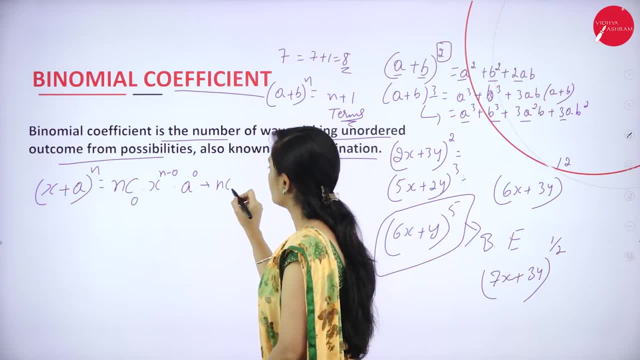 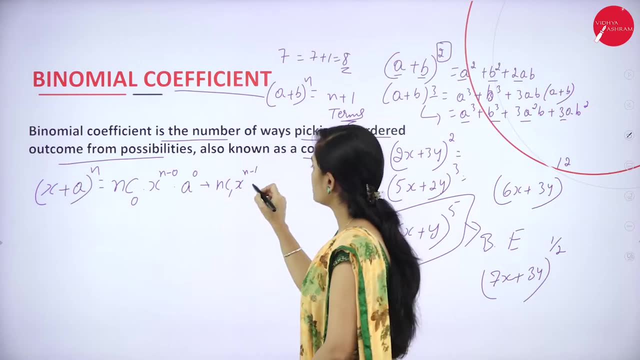 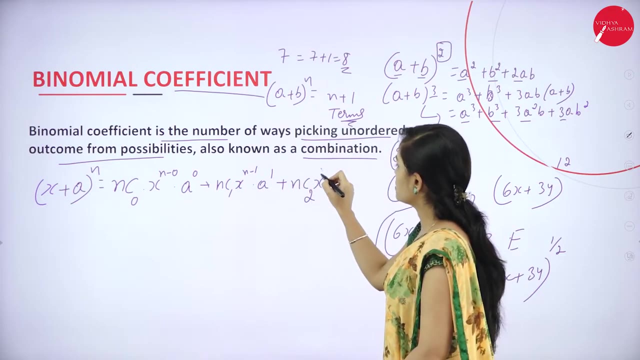 nc 0.. 0 increment is nc 1.. And what is the difference x power, n minus 1.. And 0, 1 increment means it is a power 1. And nc 2.. And what is the difference? n minus 2 into a power 1 increment is. 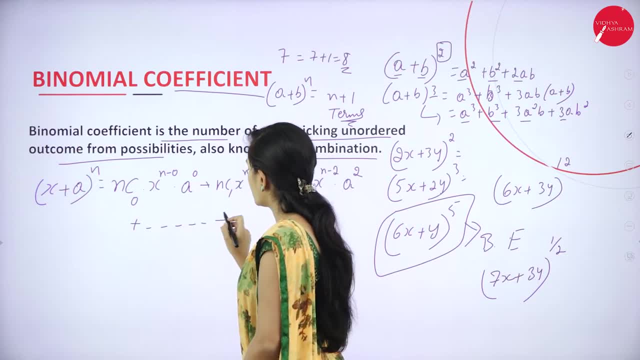 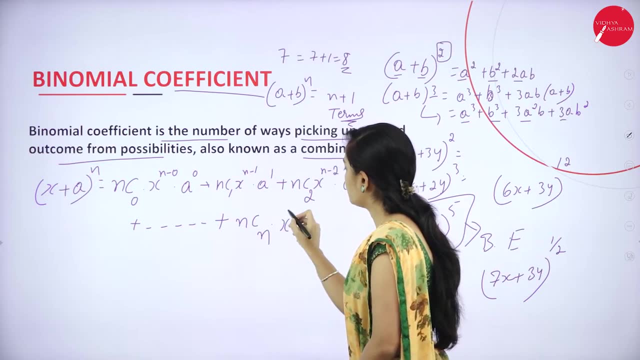 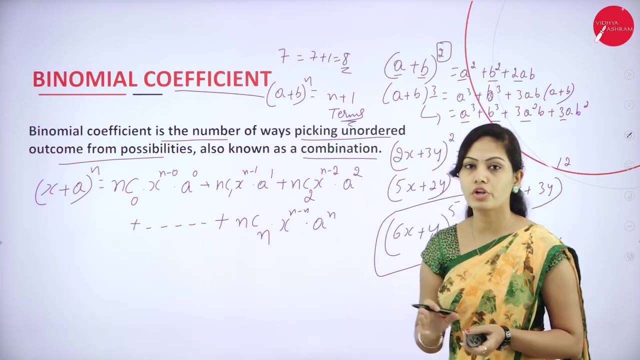 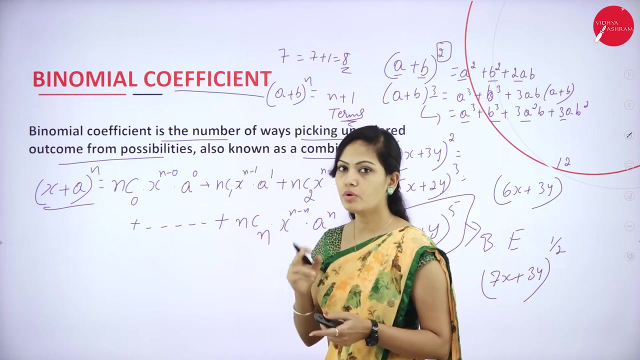 2. Plus dash, dash, dash, up to ncn, ncn And x power, n minus n into a power n. So this is the formula for binomial expansion. Here we have x plus a whole power n. If your power value is n, you will get n plus 1 terms, And I will expand. 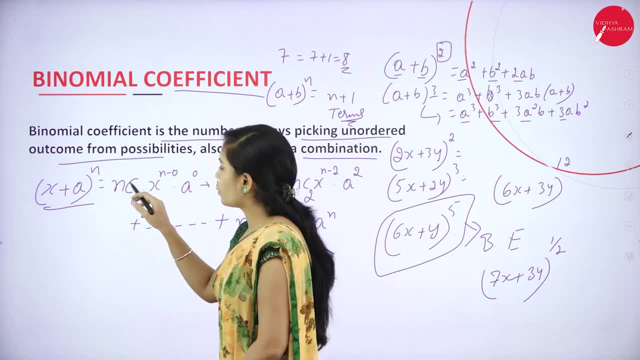 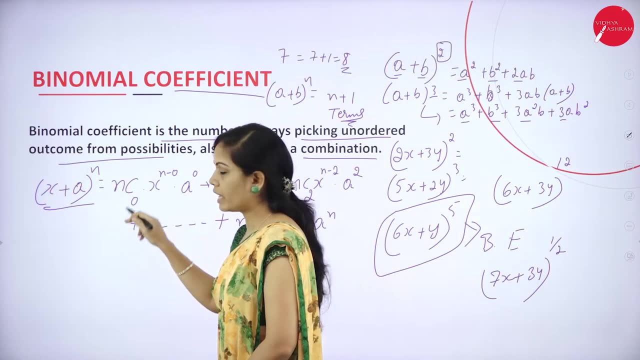 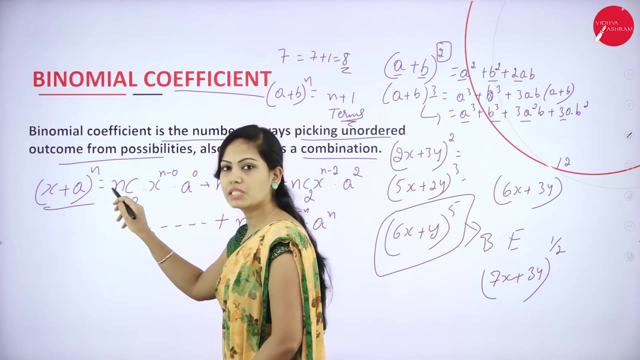 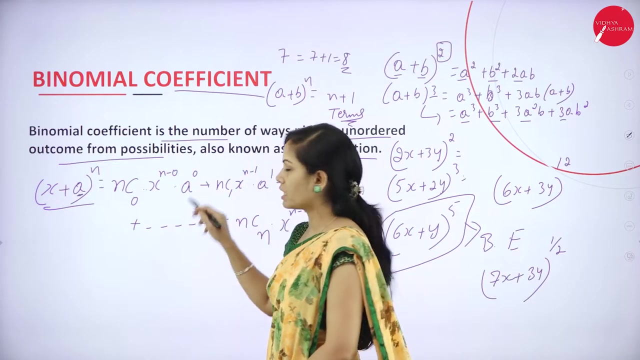 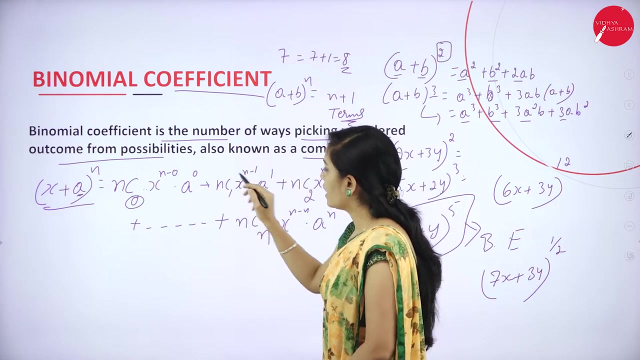 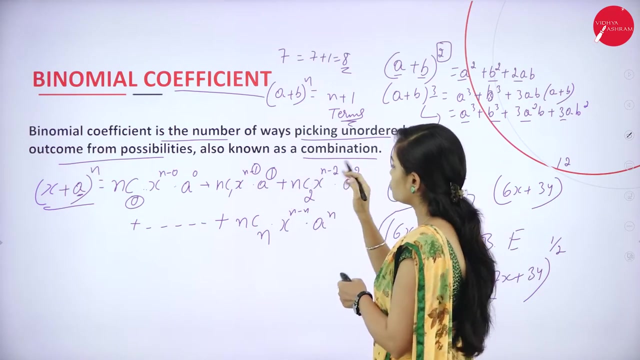 this by using combination formula nc 0. So I am applying combination formula ncr. So in place of r, I will start from initial value: 0.. nc 0.. nc 0 into x value power: n minus 0. So difference of this: nc 0 is n minus 0 into a value, a value is 0.. I will start from initial value Plus 0 is incremented by 1.. So nc 1 and 0 changes to 1 and 0 changes to 1.. So in next term, 1 changes to 2.. So 1 increment in every term. So this is the difference. 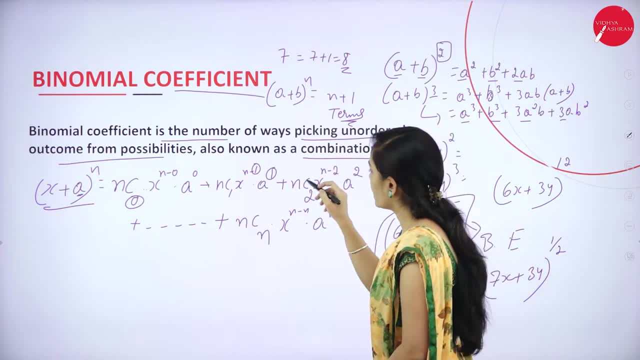 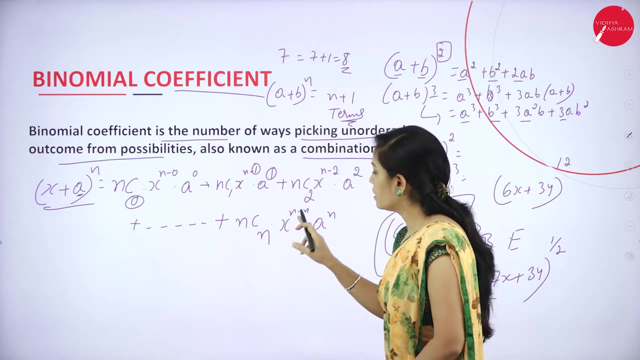 So nc 1 changes to nc 2. And x power n minus 2.. Difference of this And a power 1 changes to a power 2.. So like that, nc 3 x power n minus 3 into a power 3.. Plus dash, dash up to ncn x power n minus 1- into a power n. So this is the expansion of binomial coefficient. 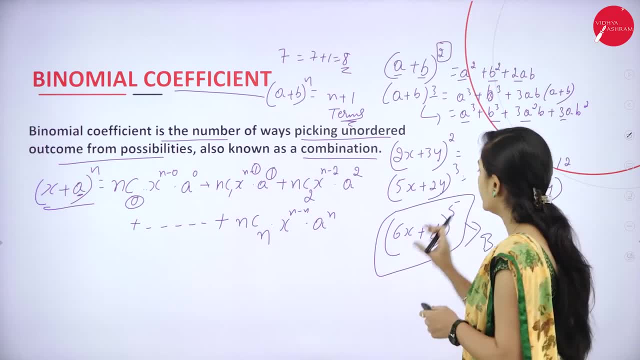 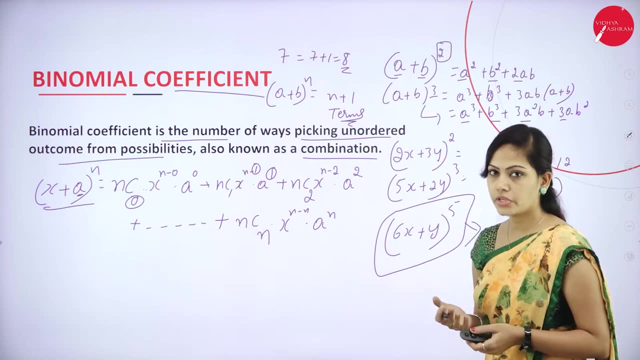 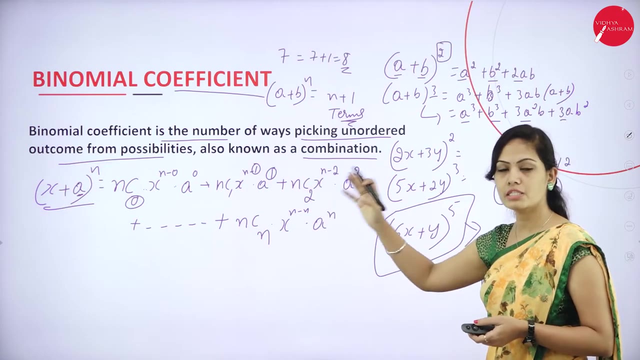 Please remember this concept, Please remember the formula You have to apply while doing the problems. If you get the power value is more than 2 or 3, or if you get fractional part, or if you get the root values, So easily, you can simplify by using this binomial coefficient. 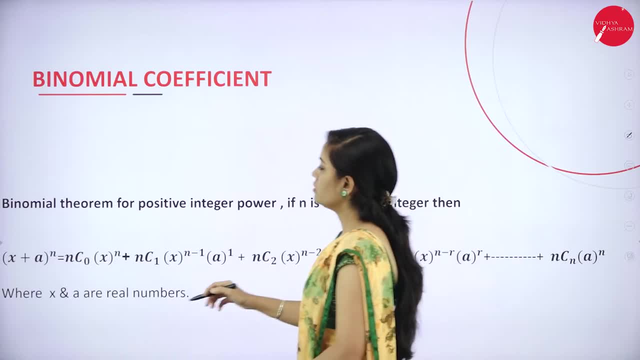 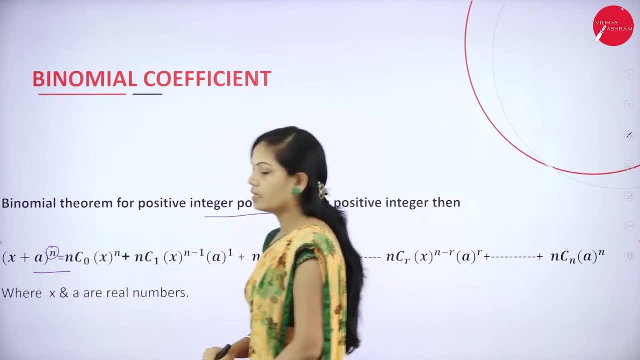 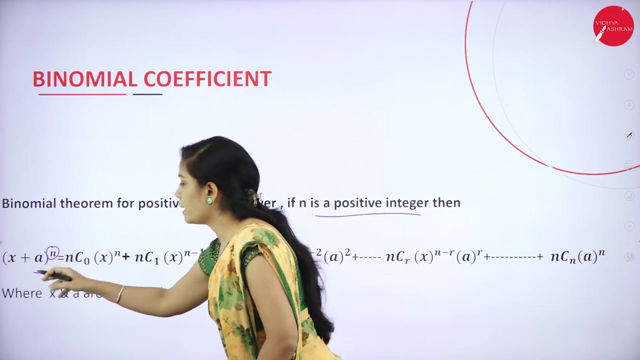 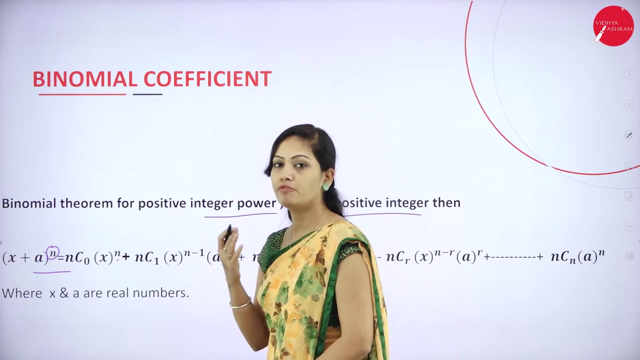 or binomial expansion. So the formula binomial theorem for positive integer power. So power value is n. n means positive integer. If n is a positive integer, then what is the formula? x plus a power n is equal to nc 0, x power n into a power 0.. A power 0 means power. if your power 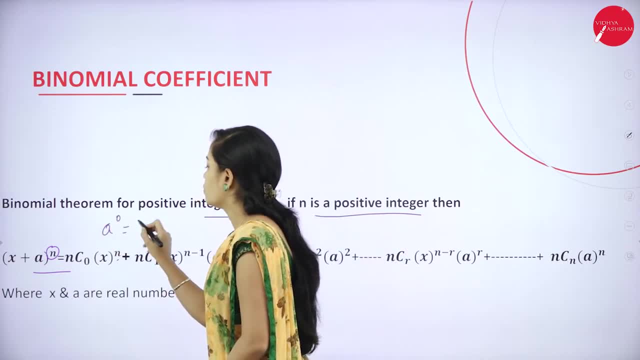 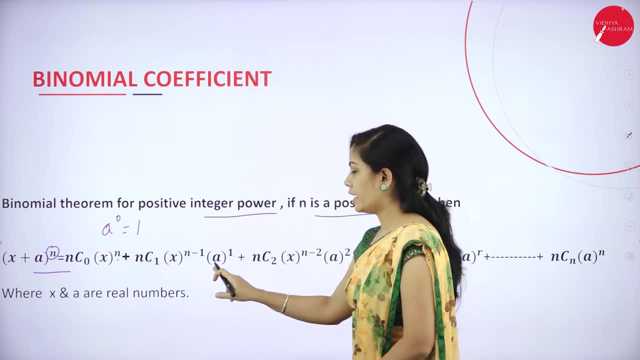 value 0 means it is always equal to 1.. So 1 means directly. you can write: it is a power 0. And a power 0 changes to a power 1.. A power 1 changes to a power 2.. A power 2 to a power r up to a power n. 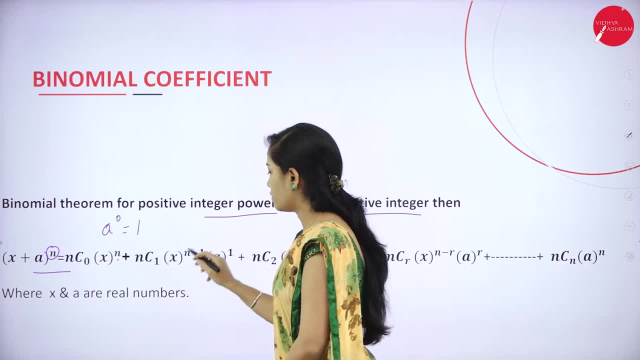 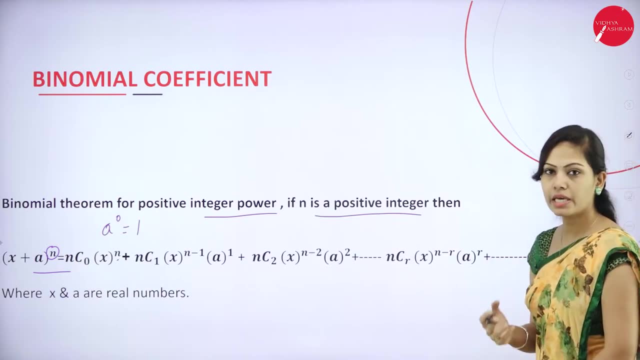 And x power n. x power n minus 1, x power n minus 1.. So this is the expansion of binomial coefficient n minus 2, x power n minus are up to x power n minus n. n minus n means it is 0.. So x power 0. 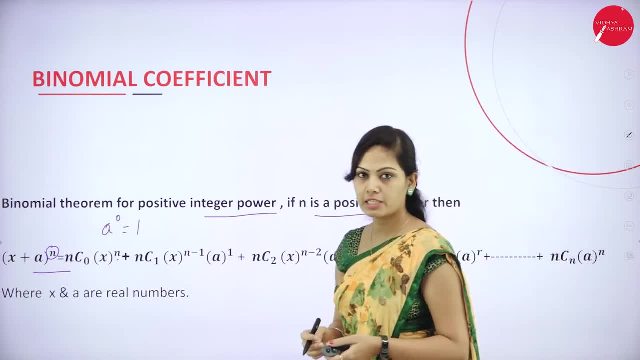 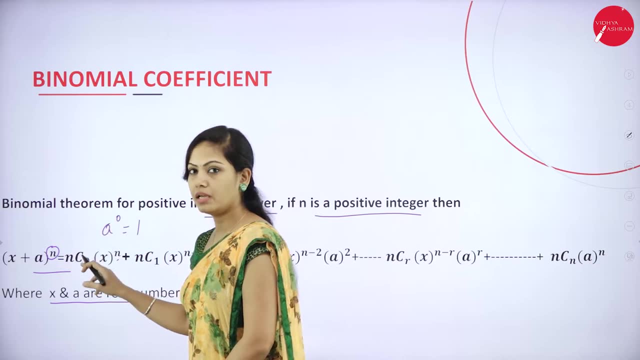 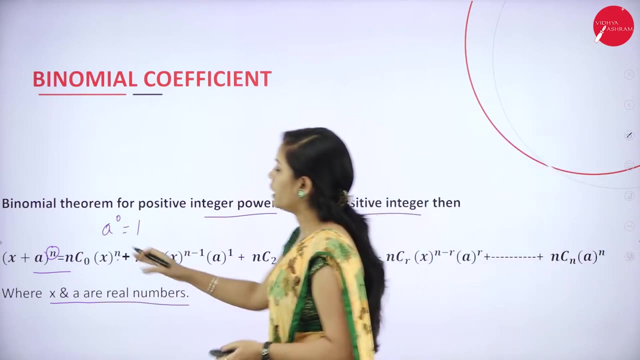 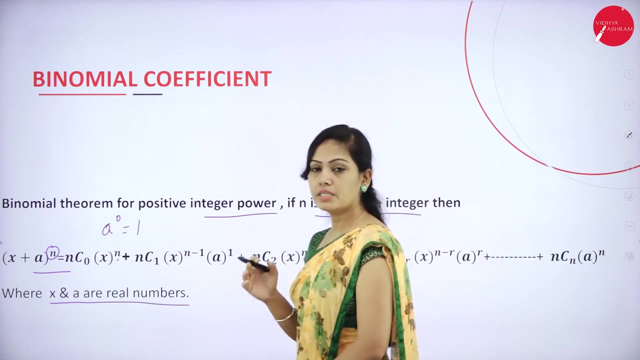 means it is 1.. So this is the formula for binomial expansion, where x and a are real numbers. So here in expression I have x plus a, So x and a are real numbers. So here we have combination formula: nc0, nc1, nc2, nc3, etc. up to ncn. Every time we can't apply this combination formula. Example: if 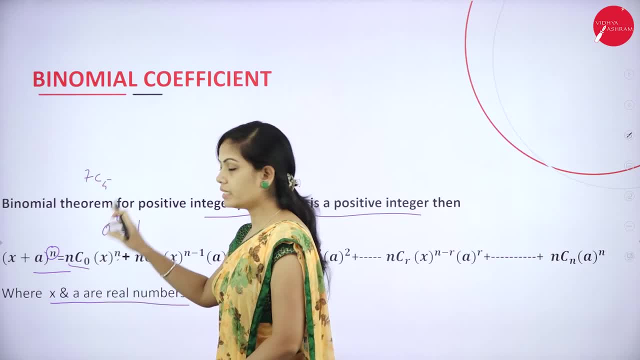 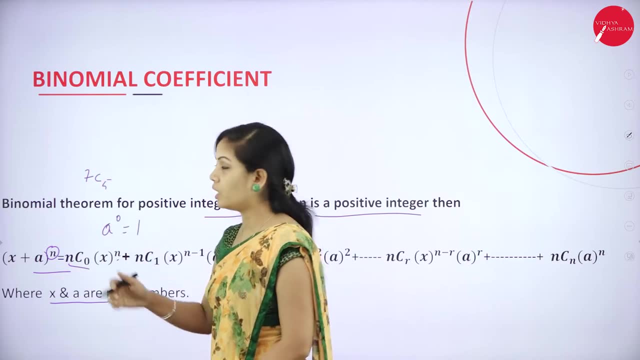 your nc0 value is 7c5.. Assume that if your nc0 value is 7c5, you have to find the value of 7c5.. You have to apply the formula called n factorial by n minus r factorial into r factorial In next. 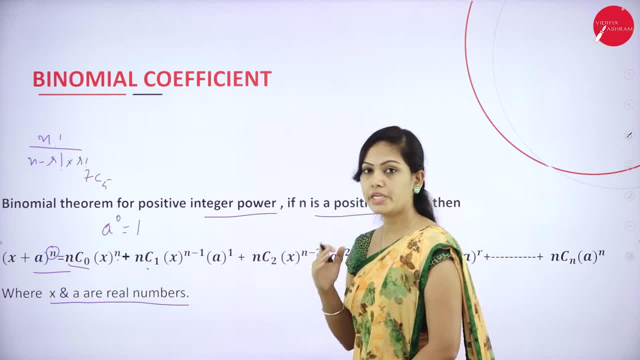 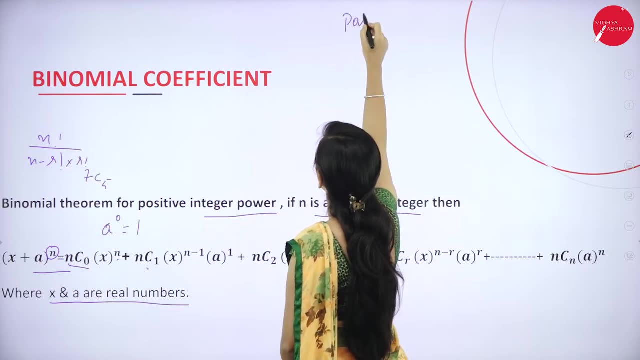 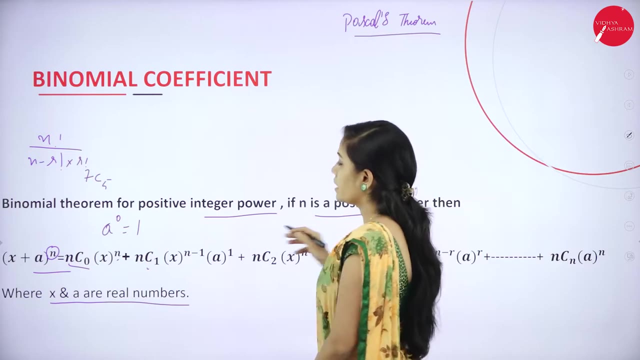 term, you will get 7c6 and 7c7.. Every time you can't apply this formula, So for that we are using Pascal's theorem, Pascal's theorem. By using this Pascal's theorem, easily we can find the combination like 7c5.. If. 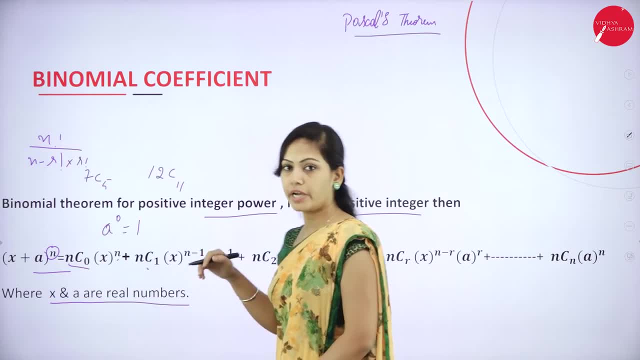 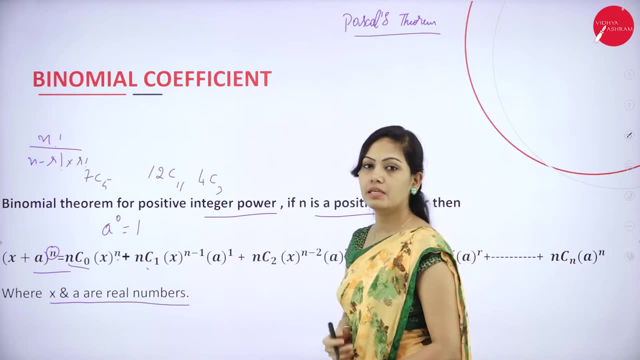 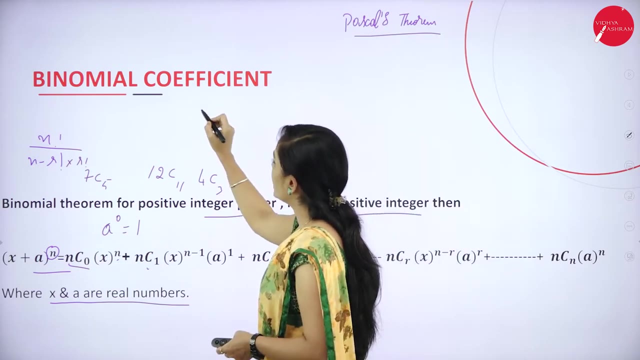 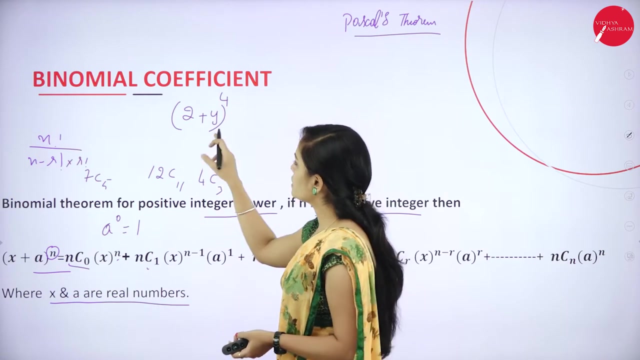 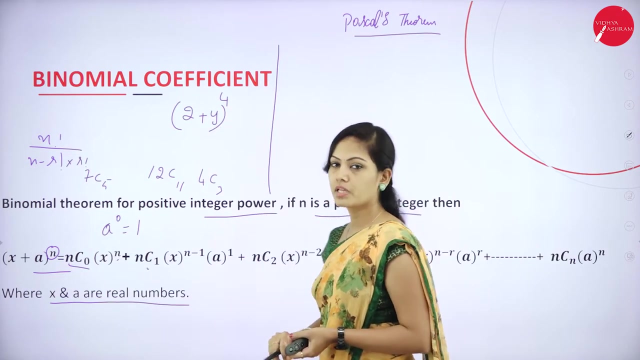 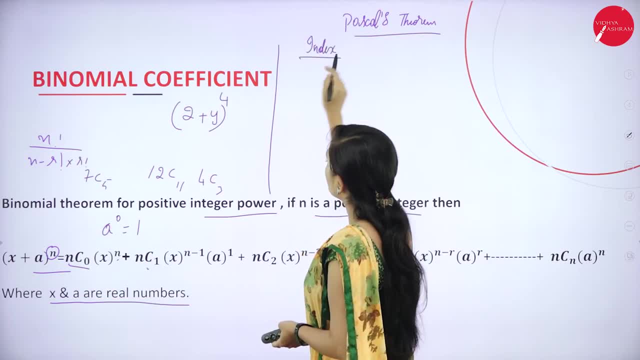 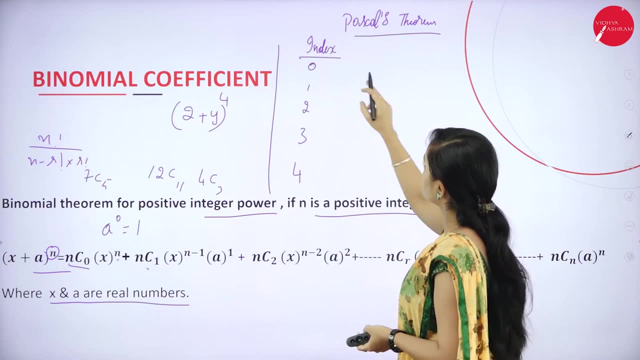 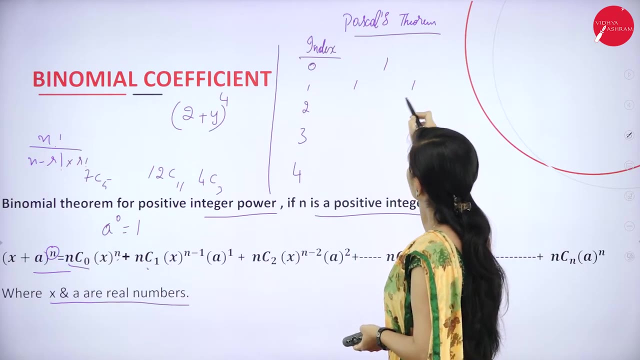 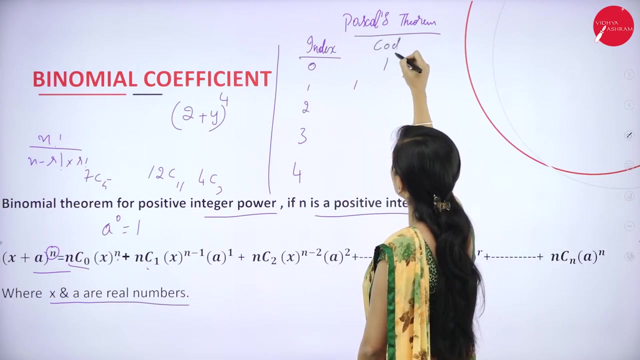 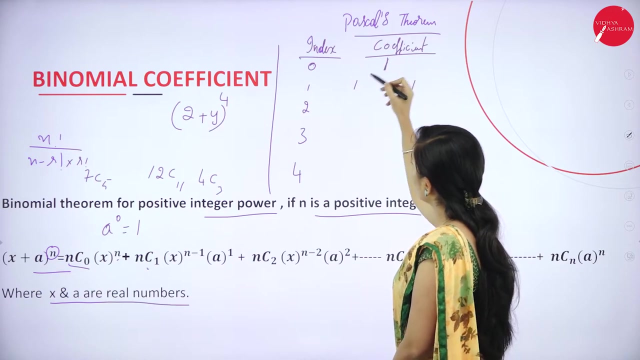 is, index value starts from 0,, 1,, 2,, 3 and 4. so now, if your index value is 0, then it's 1 clear, and again I'm using Pascal's theorem. so if your index value is 0, coefficient value is 1 clear. I starts from 1 and 1, 1, 1. I will start from 1, 1, 1. 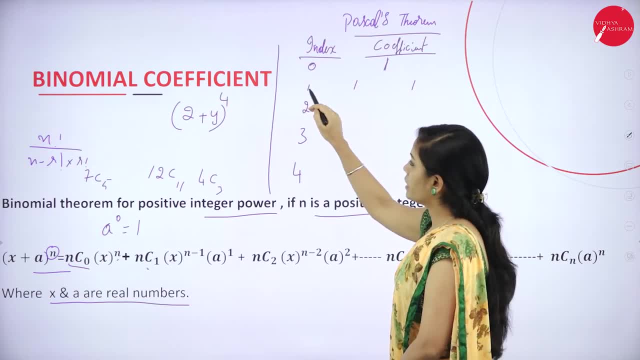 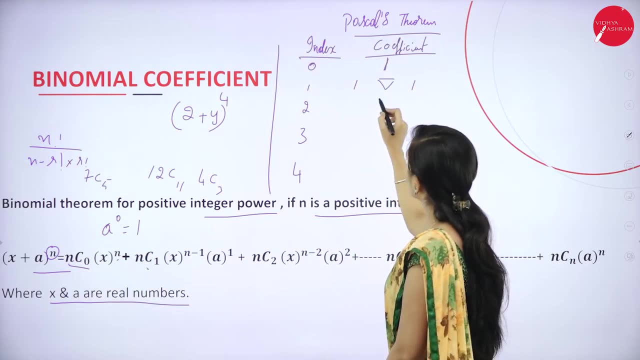 if your index value is 0, it is 1, and index value is 1, it is 1, 1 that is 2, and I'm using Pascal's theorem. so 1 plus 1 is 2, again same 1. I'll write the coefficient. 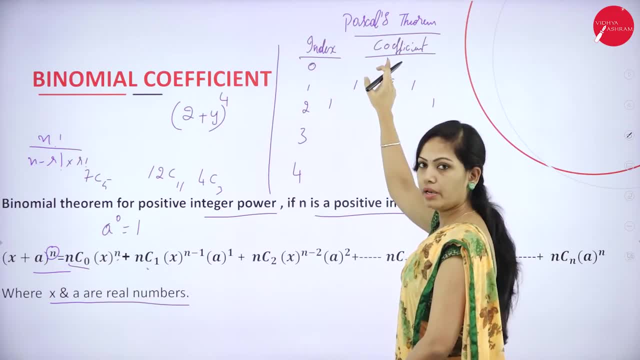 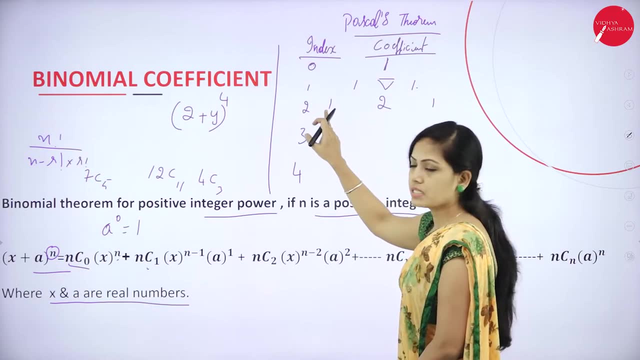 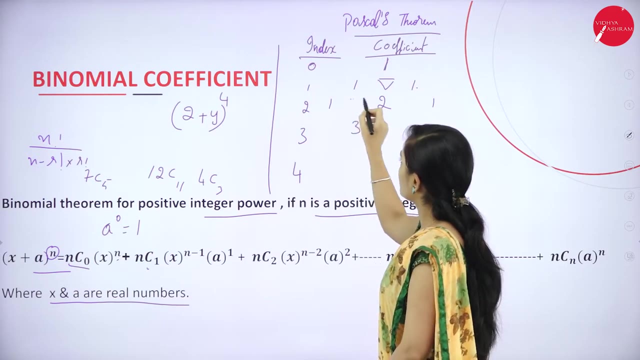 part. so I'll repeat, I'll start from 1,, 1, 1, and I'm applying Pascal's theorem: 1 plus 1 is 2. so again as it is, i'll write 1, and here also i'll write 1, and now 2 plus 1 is 3, Pascal's. 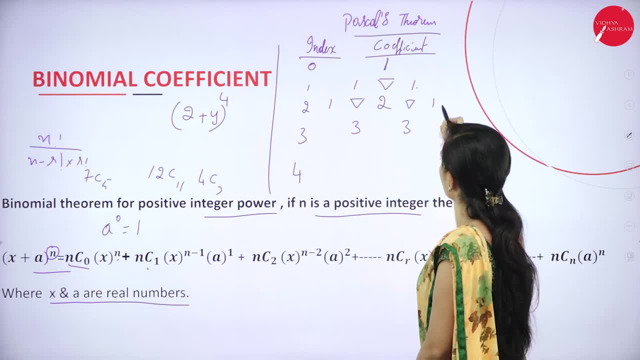 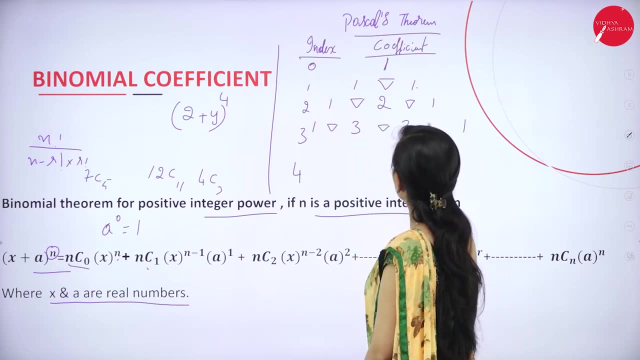 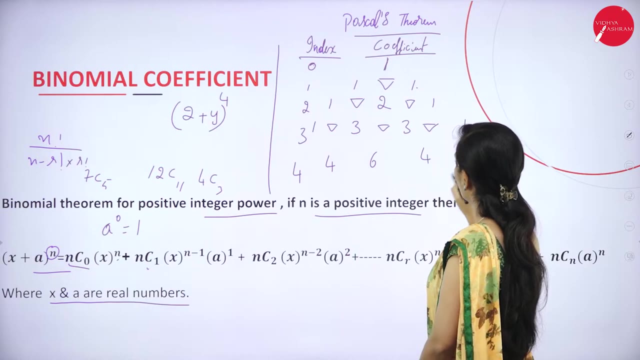 theorem: and 2 plus 1 is 3, so as it is 1, i'm writing here and one clear and again i'll apply: 3 plus 1 is 3, 4, 3 plus 3 is 6,, 3 plus 1 is 4.. So, as it is, I will write 1 and here 1.. So again, I will apply. 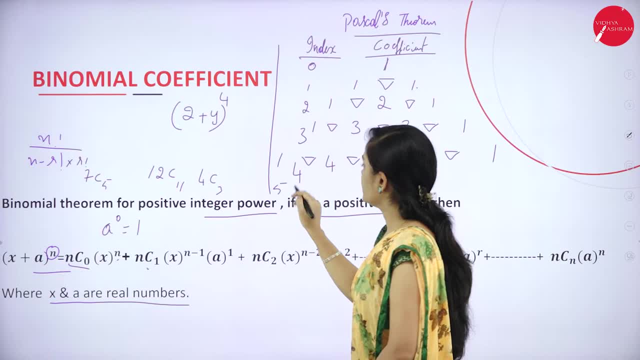 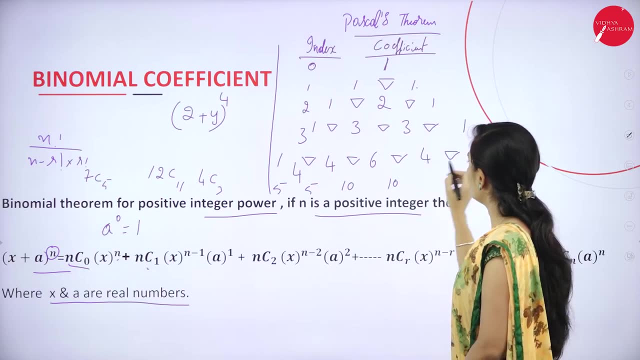 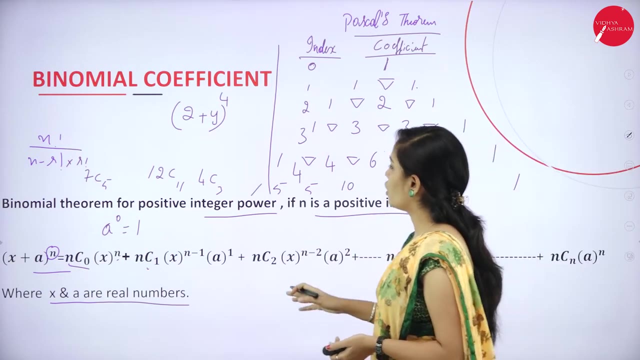 Pascal's theorem for index value is 5.. So 4 plus 1 is 5, 4 plus 6 is 10, 6 plus 4, 10, 4 plus 4, 4 plus 1: 5. again as it is, I will write 1.. So like that you can find the value of 4c3. 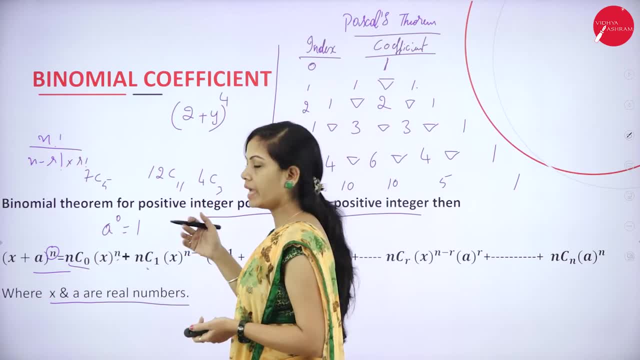 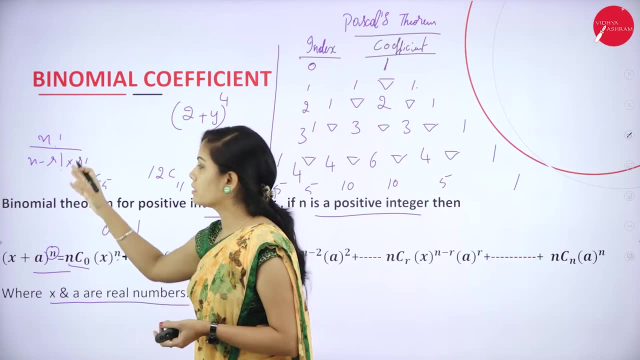 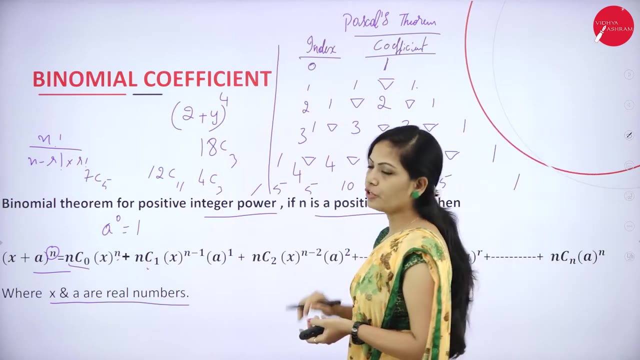 12c1,, 12c7,, 12c8 and 18c3 for every time. no need to find, no need to apply this NCR formula. So by using Pascal's theorem, easily you can find the value of 0,, 1,, 2,, 3,, 4, etc. 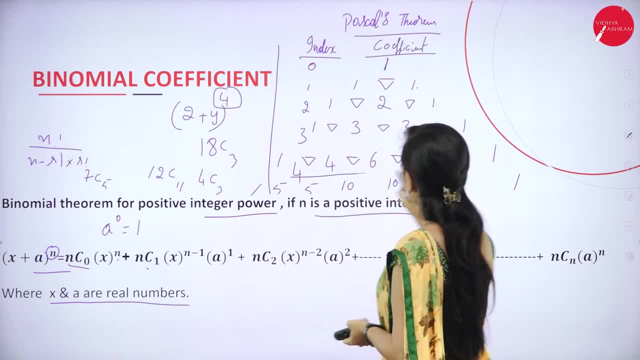 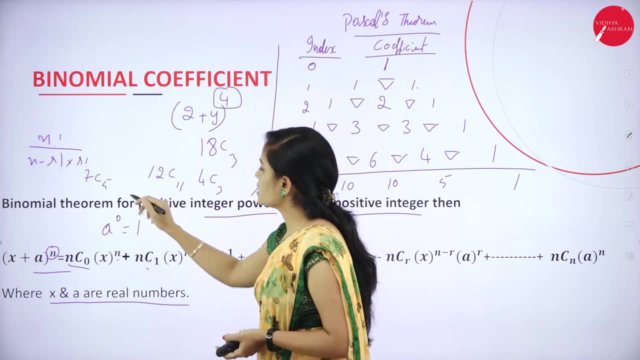 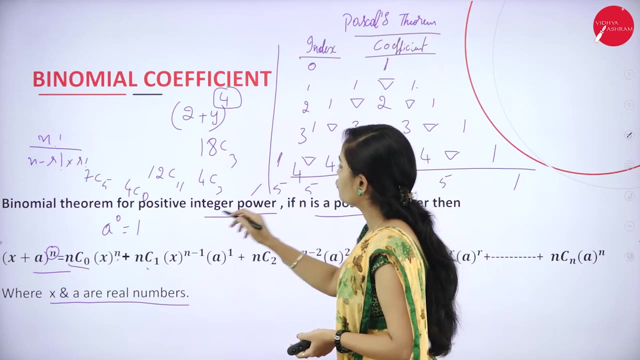 If your power value is 4, so till here you can use the values. So 4 means if your power value is 4 means So it is 4c0.. 4c0 means it is 1.. You can find out, and for in next step you will get 4c1.. So 4c1. 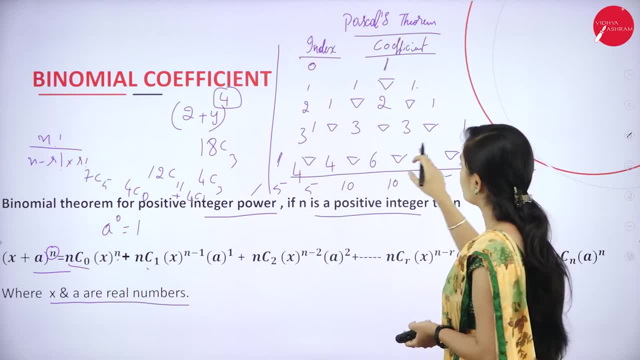 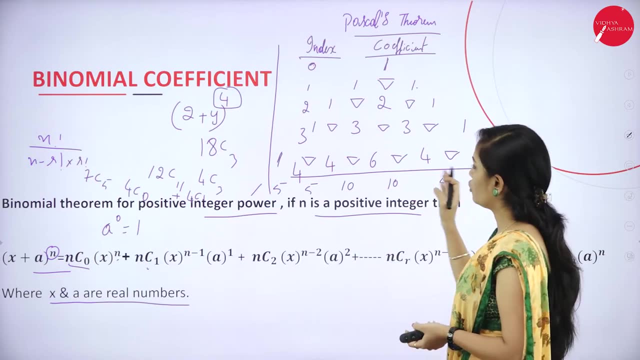 value is 4 and 4c2 value is 6.. 4c3 is 4 and 4c4 is 1.. Like that, you can easily, you can find the value of combinations by using Pascal's theorem. Now, this is the binomial expansion formula. 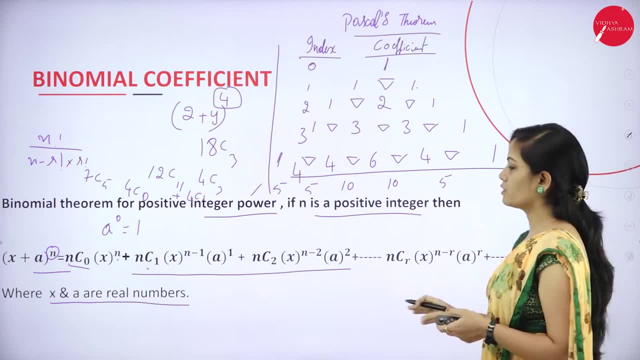 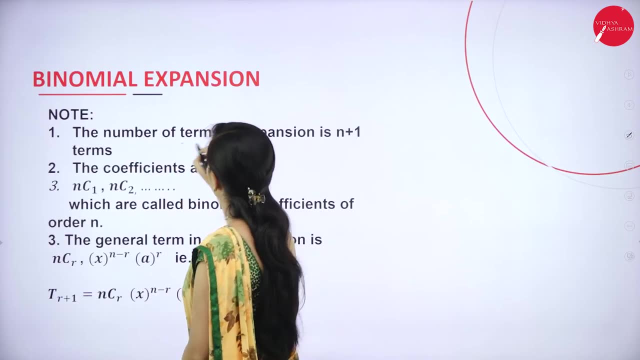 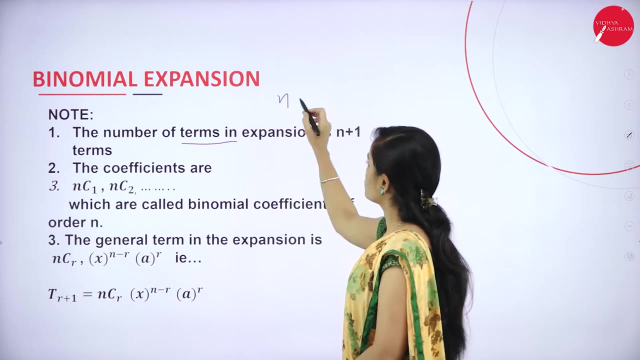 Please remember this. It is very important. by using this formula easily, we can simplify binomial expansion. and next one: binomial expansion: The number of terms in expansion is n plus 1 term. So already I have told you, if you, if your power value is n, So the terms is n plus 1 terms. and the second point: 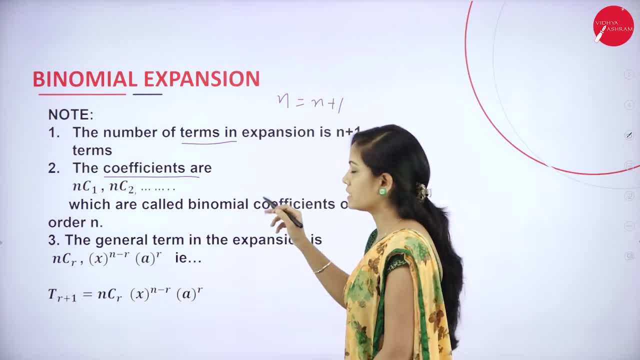 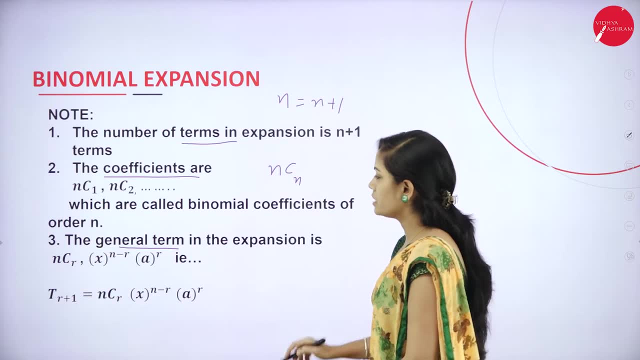 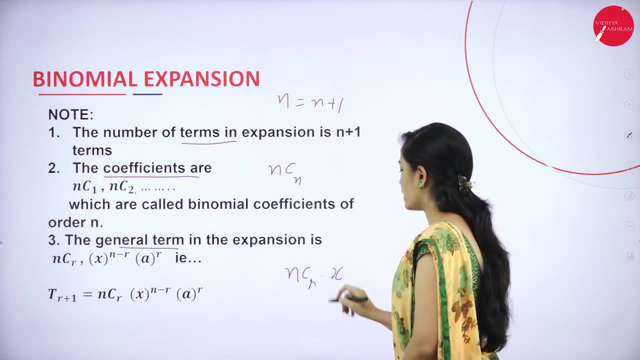 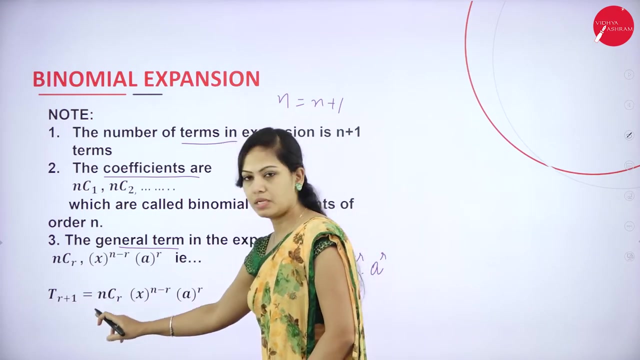 the coefficients are nc1, nc2, nc3 up to ncn and the third step, The general term in the expansion, is ncr. If it is, ncr means the power value is difference, is n minus r, x, power n minus r into a power r, That is tr plus 1.. tr plus 1 means the next term. tr plus 1 means 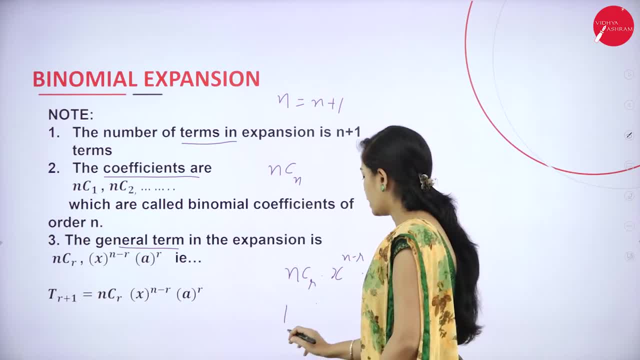 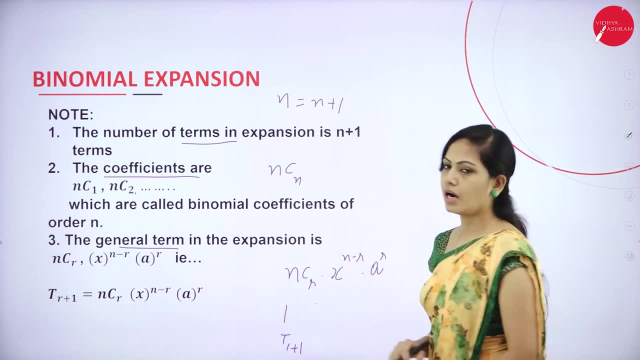 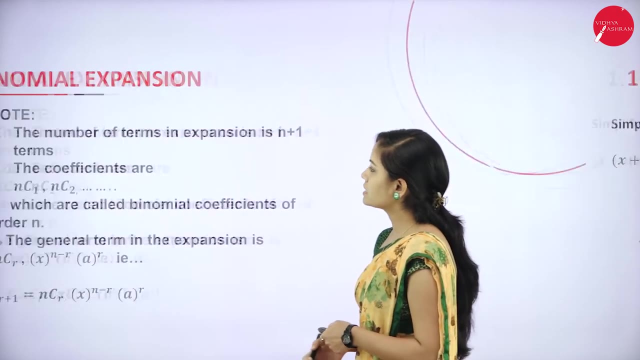 if your r value is 1.. So tr plus 1 means 1 plus 1.. Clear So ncr into expansion, So ncr into a power n minus r into a power r. So by using this formula- expansion formula, easily we can simplify the binomial expansion. Let us understand with an example problem. It is 7 marks. 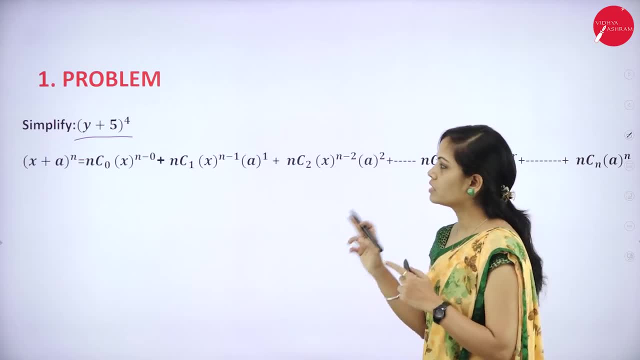 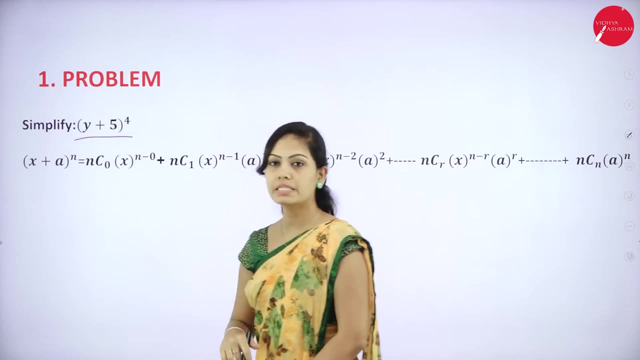 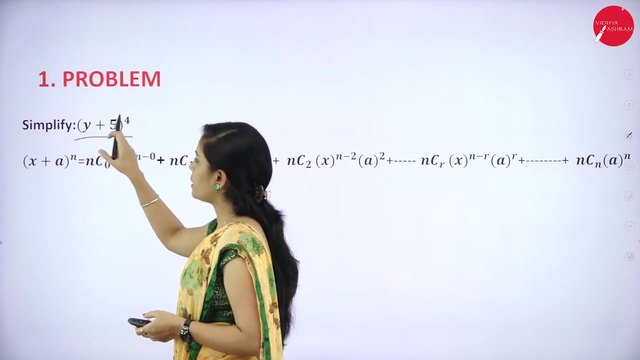 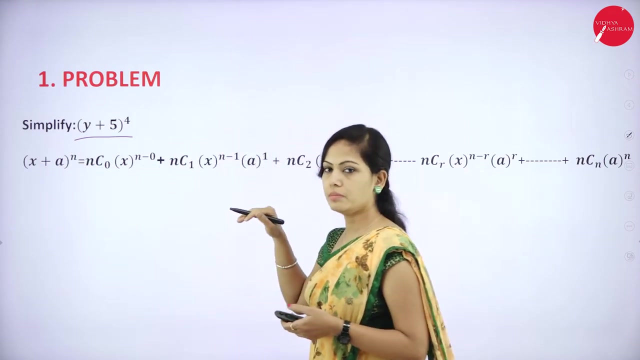 question. Definitely, definitely, there will be a problem on this concept. binomial expansion: So here we have an expression. You have to expand this expression by using binomial coefficient concept. So here, just observe this, We have y plus 5.. So what is the formula? x plus a power n. So this is the binomial expansion. 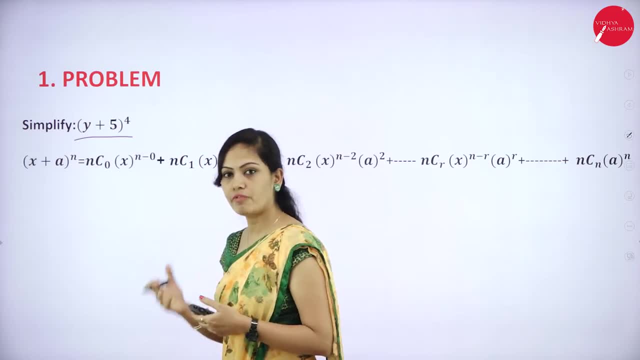 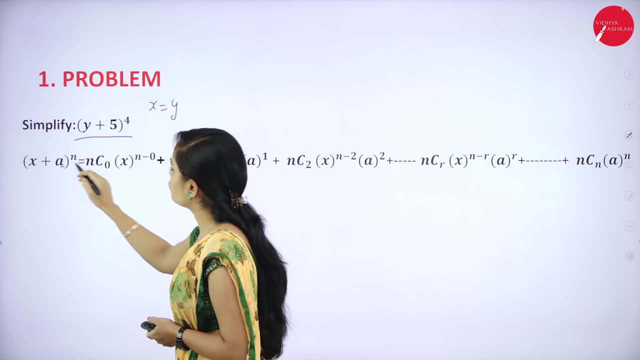 By using this binomial expansion, we can expand this and we can find the value. In place of x, I have y, So x is equal to what y, And in place of a, I have 5. So a is equal to 5.. 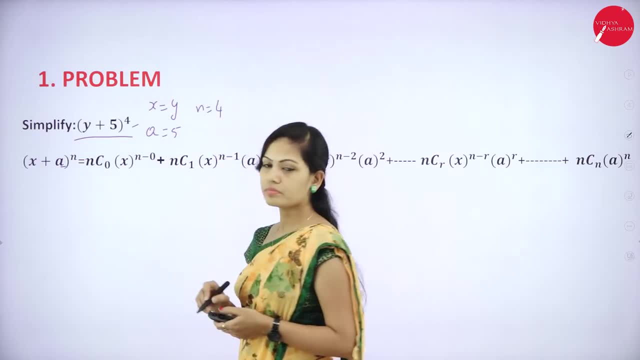 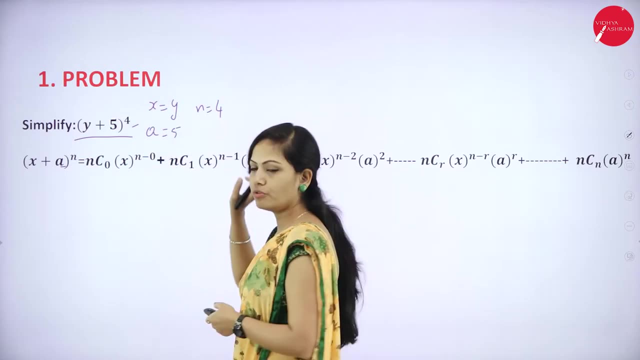 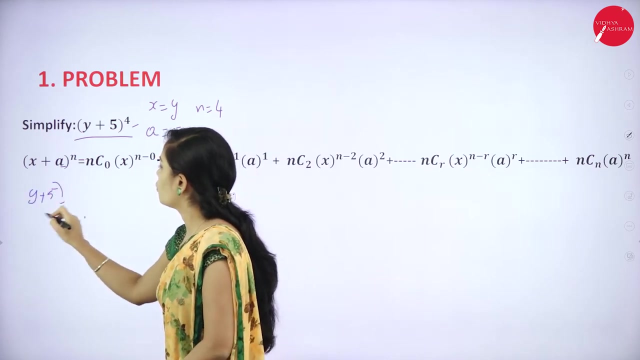 And in place of n I have 4.. So first write the given values. x is equal to y, a is equal to 5. n is equal to 4.. So whatever the value, the given value, you just write it: x, a and n values. So easily you can substitute the value here. So now y plus 5 whole. 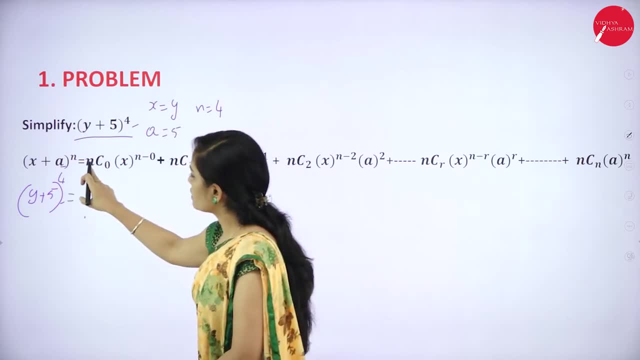 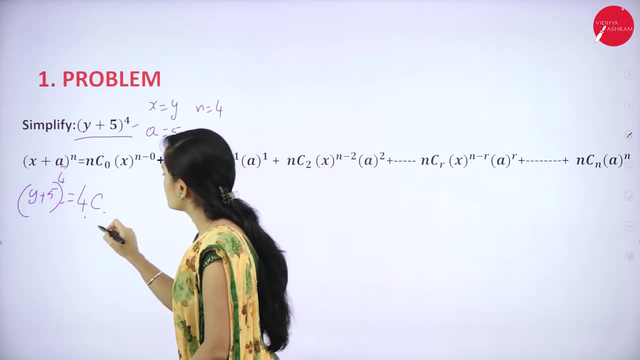 power 4 is equal to. So what is the value of n? It is 4.. c is common, That is combination, And r value is starting. So this is the binomial expansion. So this is the binomial expansion. So 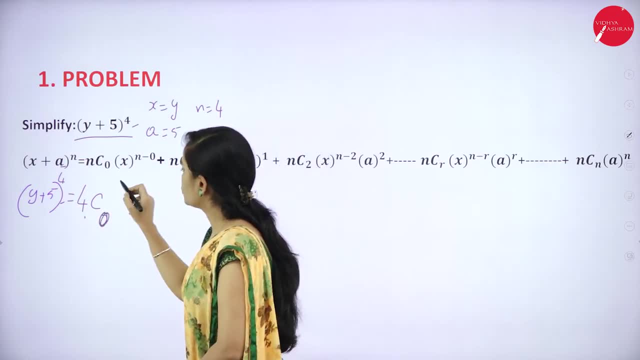 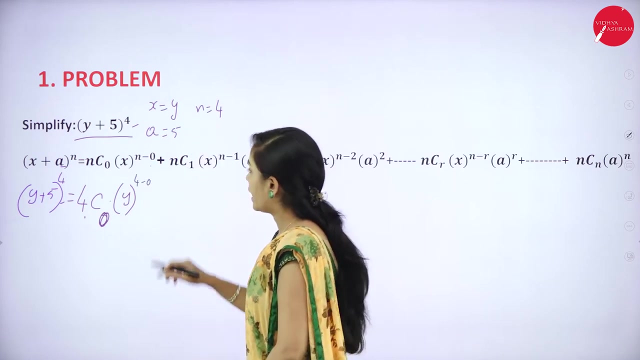 a starts from 0. So 4c 0 into x. x value means it is y y power. The difference is 4 minus 0. So here I have n minus 0. But then value is 4. So it is 4 minus 0. And next is a power 0.. If you want to write the power value, 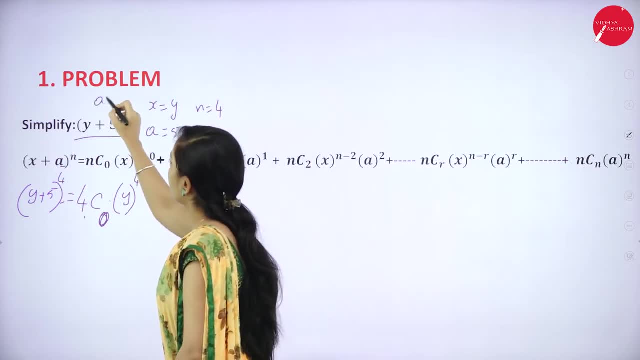 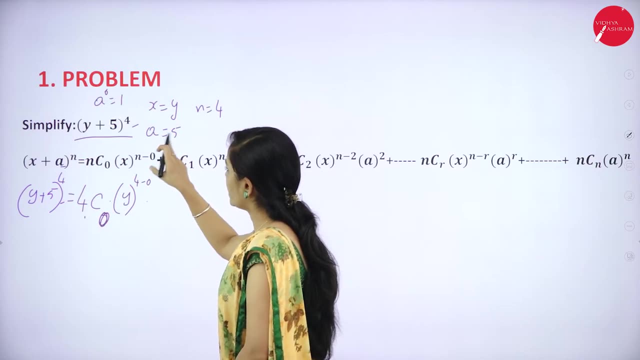 0 means it is 1.. A power o means 1.. If you want to write, you can, and otherwise you can skip because you will get 1.. 1. What is the value of a? a is equal to 5. 5. power 0 means 1.. If you want to write, you can. 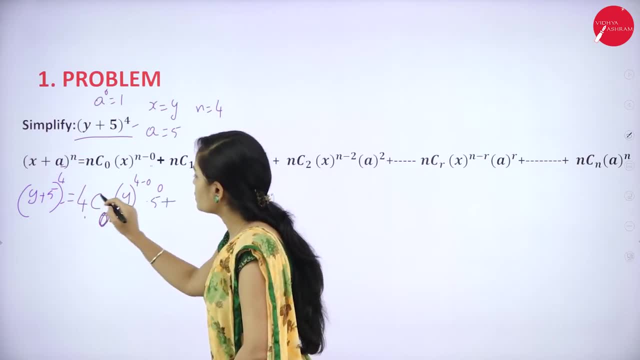 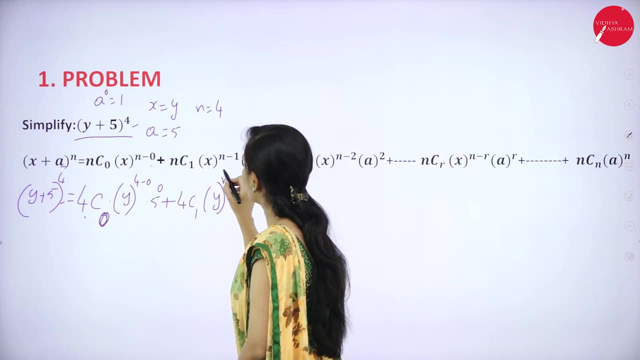 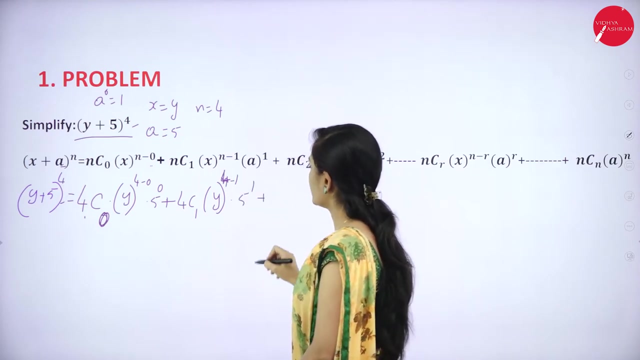 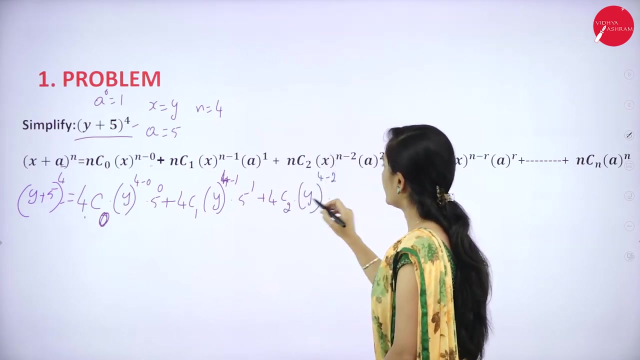 write, otherwise you can skip. and the next term 4c0 changes to 4c1 and y power n minus 1 means 4 minus 1 into a means 5. 5 power 1. and the next term 4c2- y power 4 minus 2 into a power 2. 5. 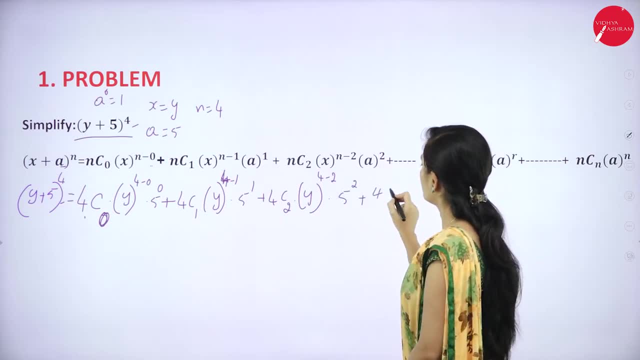 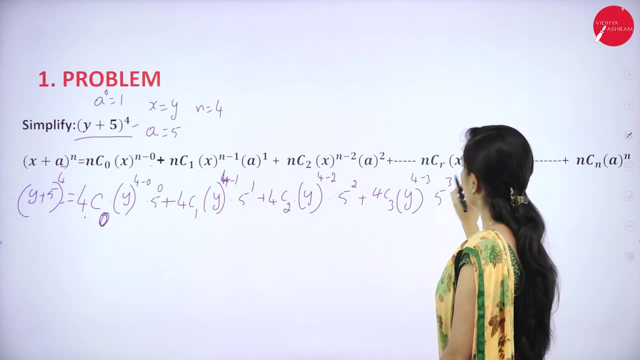 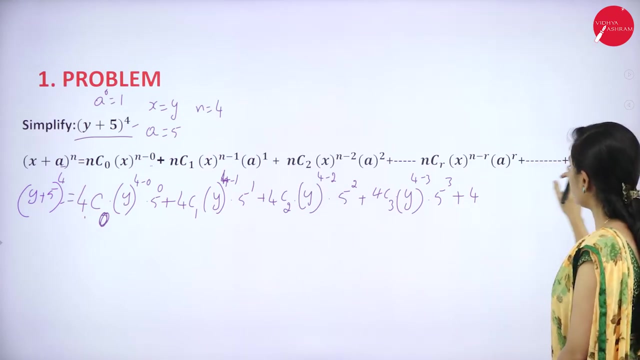 power 2 and 4c3 into y, power 4 minus 3, into 5, power 3 plus up to ncn. So ncn means the value of n and the value of r should be same. till that you have to expand the equation So 4c4. the value of n also same, the value of r also same. So till here you have to. 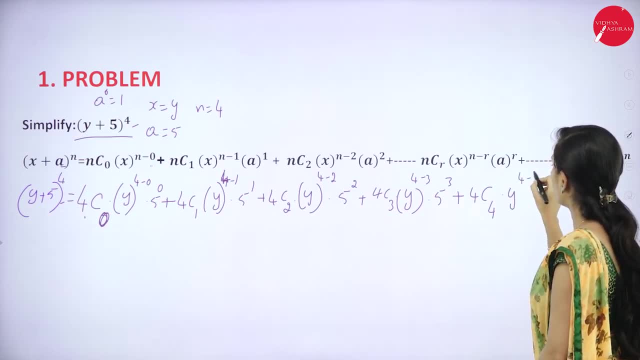 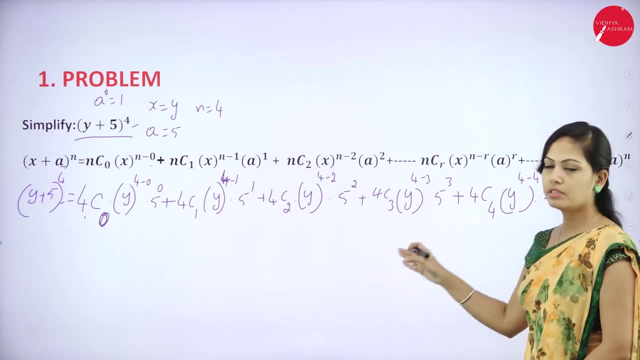 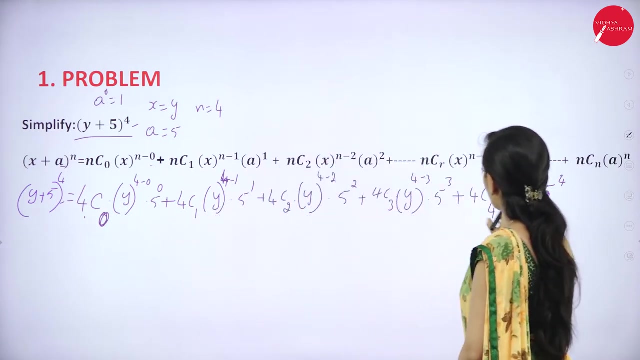 expand. So 4c4 into 4- power 4 minus 4 into 5, power 4.. So now I have expand the equation. you can observe this: How many terms are there? 1, 2, 3, 4, 5.. So if your power value is 4, you will get 5 terms, So 4c0. 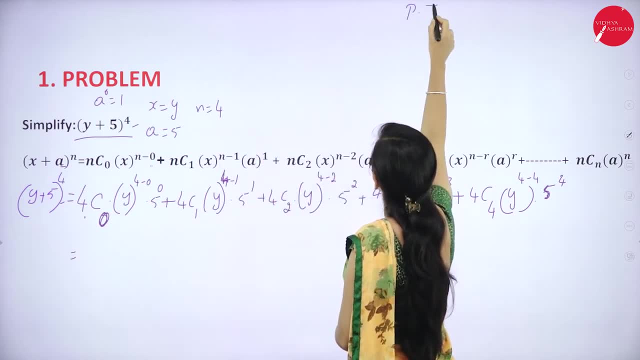 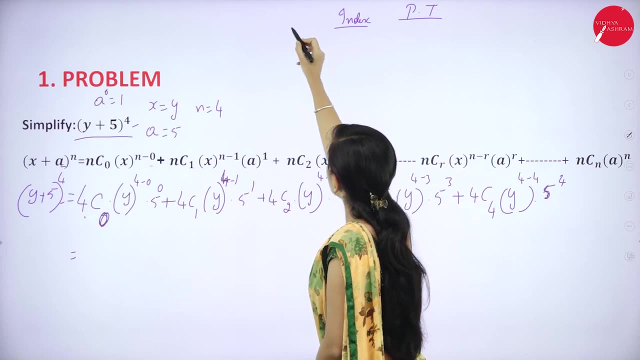 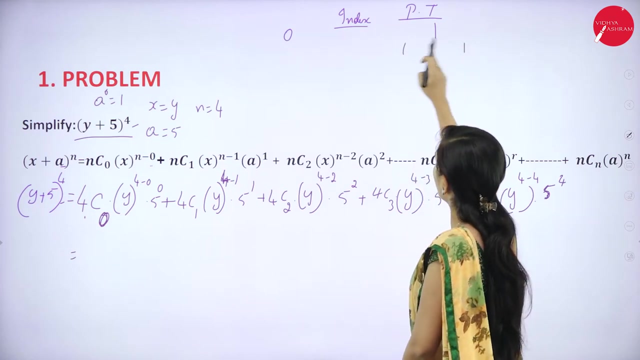 So now I will apply the Pascal's theorem. Pascal's theorem states that index value is 0 and the coefficient is 1, and I will start from 1, 1, 1, 1,, 1,, 1, 1.. So I will start from 1, 1, 1, 1, 1, 1.. So I will start from 1, 1, 1, 1, 1, 1.. So I will start from. 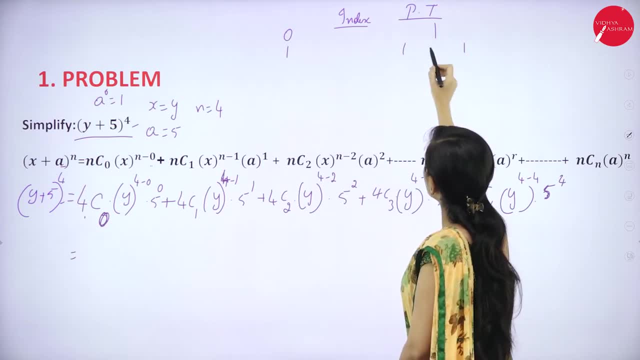 0.. So now index value is 1.. So 1 plus 1. I will add Pascal's theorem: 1 plus 1 is 2.. So this 1, I will write here. This 1, I will write here. So now the index value is 2.. 2 plus 1, I will apply 2 plus. 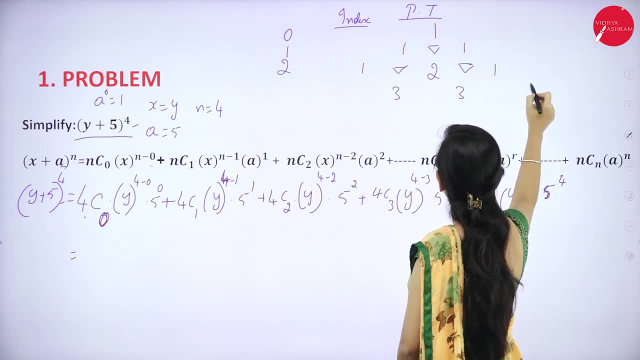 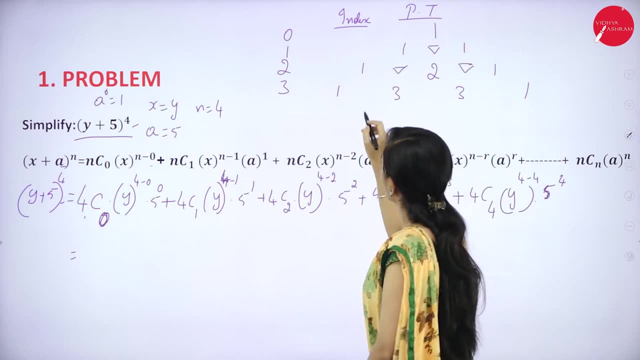 1 is 3.. 2 plus 1 is 3.. So as it is, I will write this: 1 here And the index value is 3.. So 3 plus 1 is 4.. 3 plus 3 is 6.. 3 plus 1 is 4.. As it is, I will write 1 here. So index value is 4, means 1, 4, 6, 4, 1. 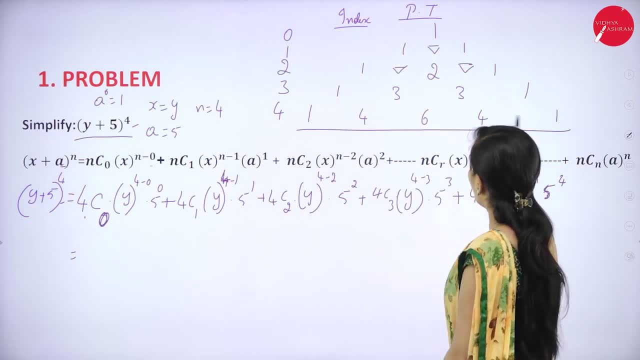 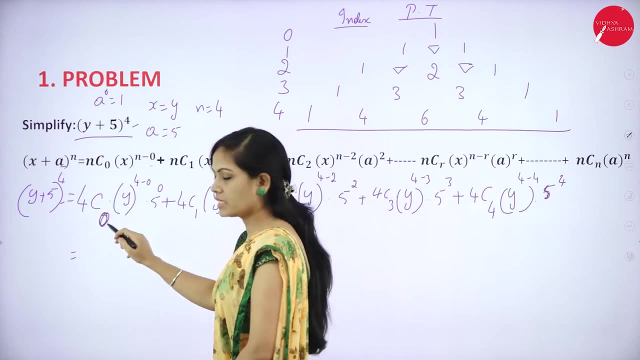 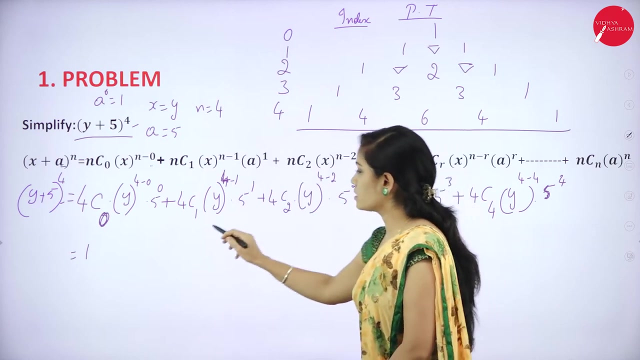 is a combination: 1, 4, 6, 4, 1.. So where you have to write this 1, 4, 6, 4, 1?? So where you have to write this: in place of 4 c 0, you can write this 1, and in place of 4 c 1, you can write this 4.. 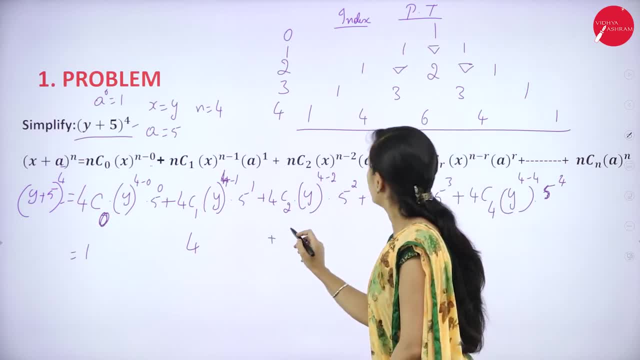 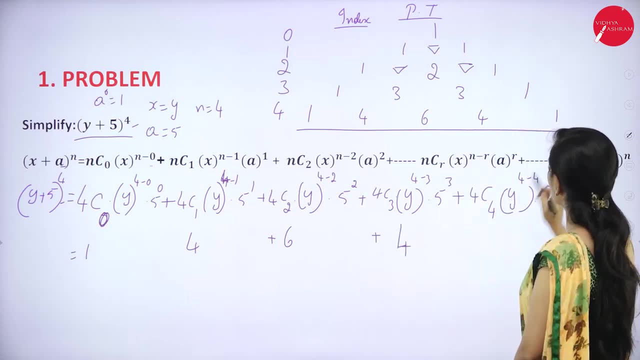 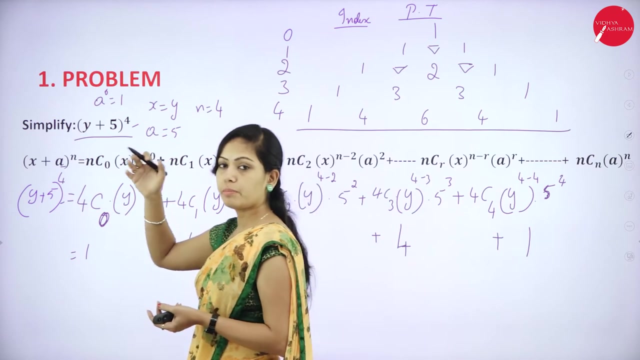 In place of 4 c 2, you can write this 6, and in place of 4 c 3, you can write this 4, and in place of 4 c 4, you can write this: 1. Clear. If you want, you can use n factorial by. 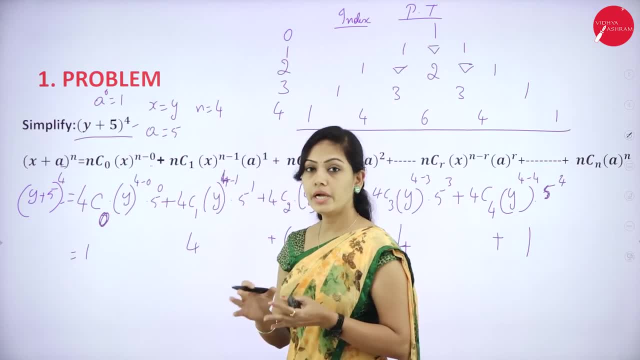 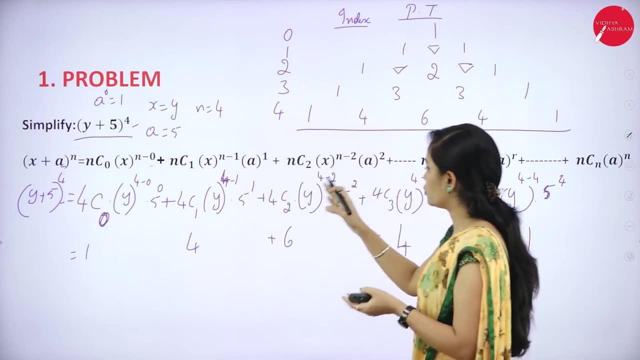 n minus r factorial into r factorial formula also. but it is very difficult. So every time you have to find out 4 c, 0, 4 c, 1, 4 c, 2, 4 c, 3, etc. So because of that, by using this Pascal theorem easily you can find out. 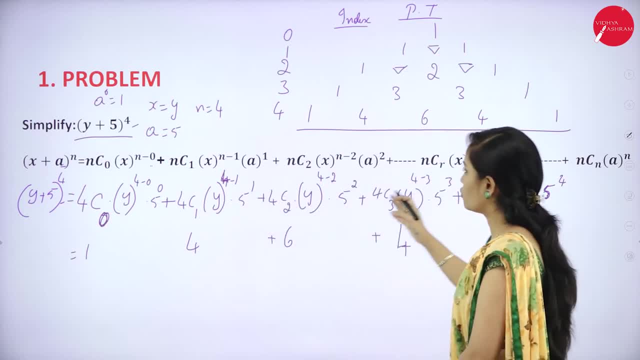 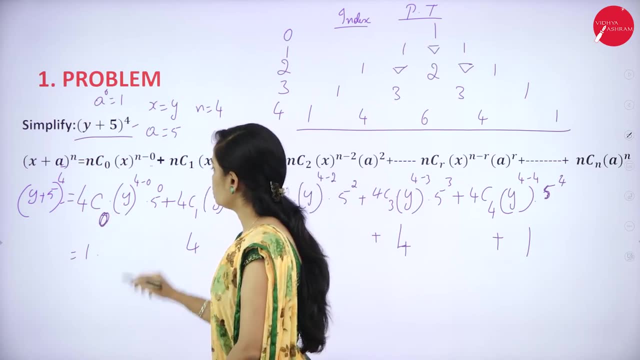 the values of 4 c 0, 4 c 1, 4 c 2, 4 c 3, etc. So now I will apply this directly. So 4 c 0 means it is 1 into y power 4 minus 0.. 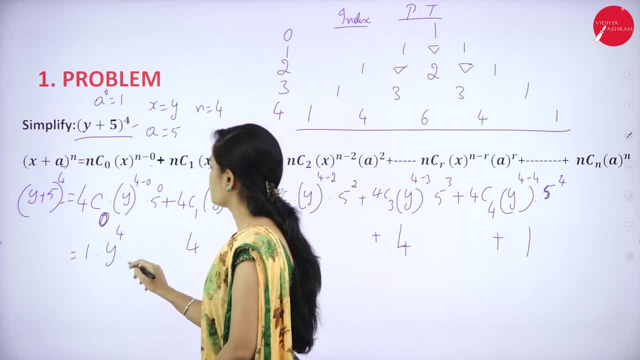 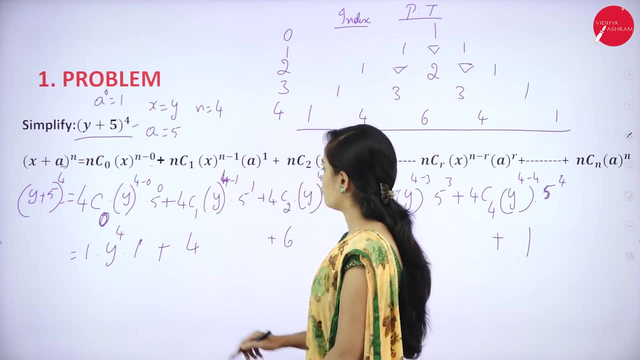 y power 4 minus 0 means it is y power 4 into 5 power 0 means it is 1.. If you want, you can write, otherwise you can skip. So 4 c 1 is 4.. So 4 minus 1.. So 4 minus 1 means it is 3.. 5 power 1 is 5. 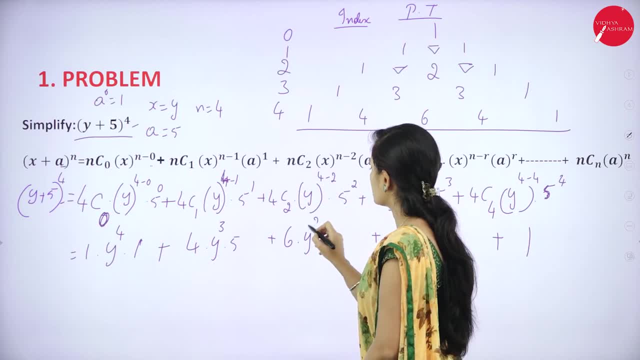 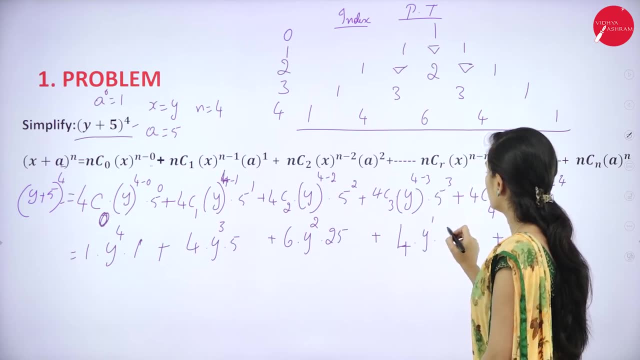 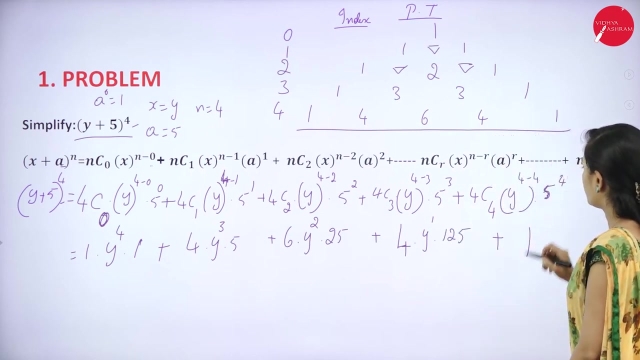 and y power 4 minus 2 is 2.. 5 square means 25 and y power 1 into 5 cube It is 125.. And y power 4 minus 4.. So 4 minus 4 means it is y power 0.. y power 0 is equal to 1.. 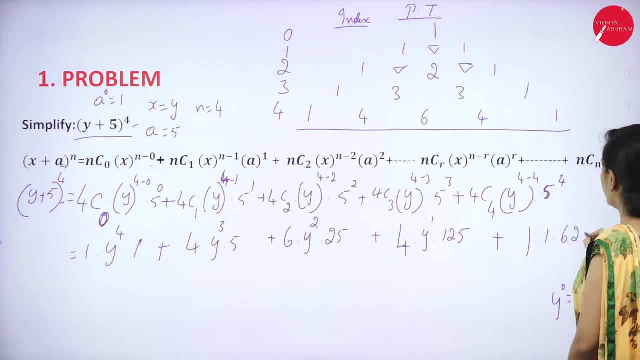 So 5 power 4 means it is 625.. You can use calculator, normal calculator. Please don't use scientific calculator. 5 power 4 means 5 into 5. into 5 into 5 will get 625.. So now you can. 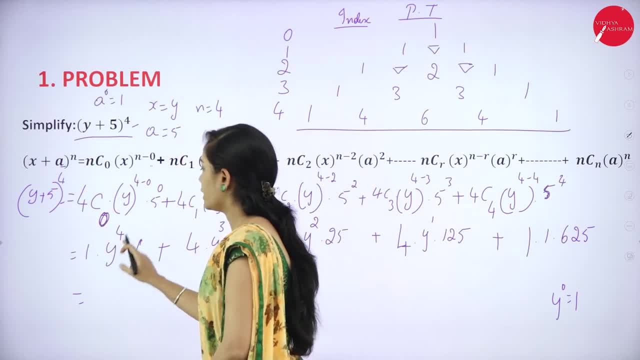 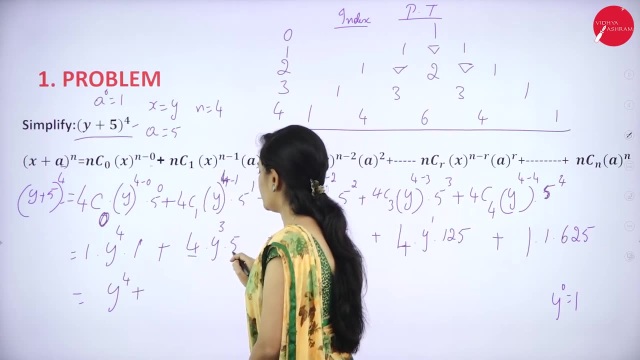 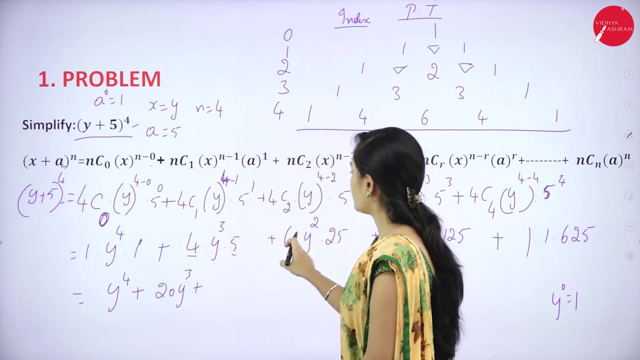 simplify this expression: 1 into y power. 4 into 1 means it is y power 4 plus 4 into y cube into 5.. 4, 5 is a 20 y power 3 and 25 into 6.. Find out 25 into 6 and write the value. 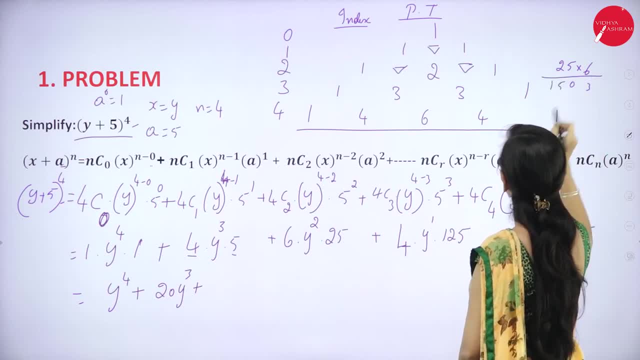 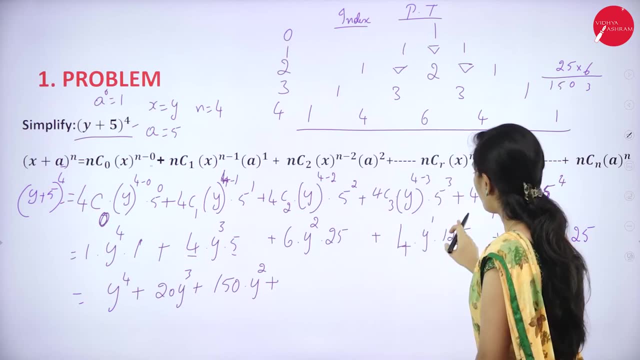 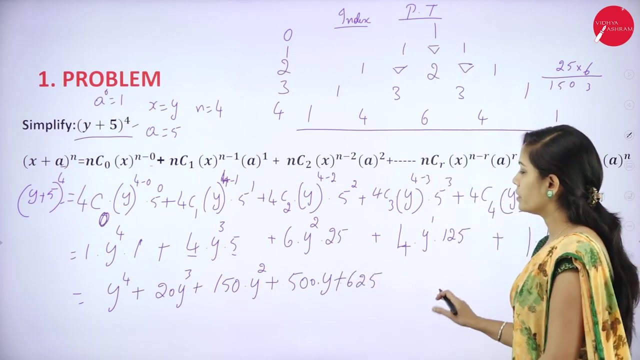 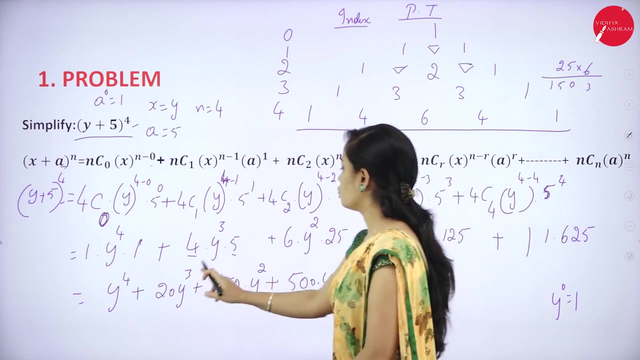 So it is 150 into 4. y square plus 125 into 4 is 500 into y. power. 1 means y, 500, y plus 625.. So this is your final expression. Your n value is 4.. So how many terms are there? 1, 2, 3, 4, 5.. 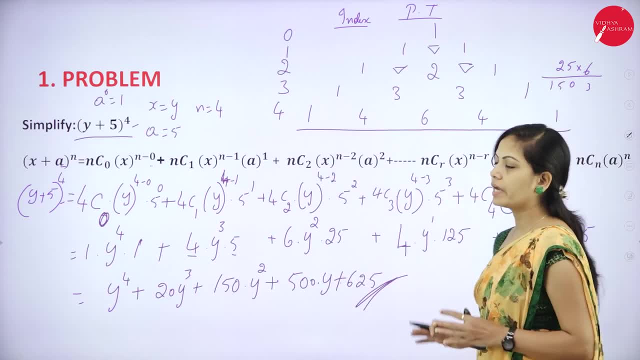 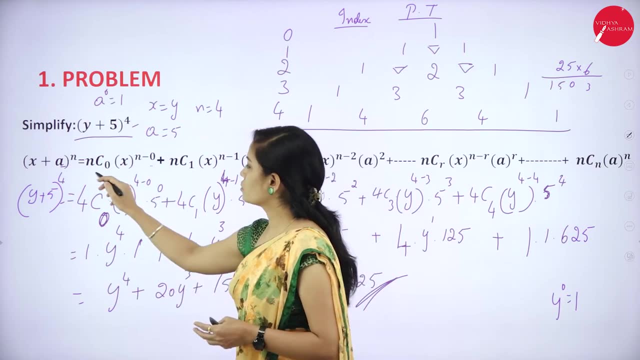 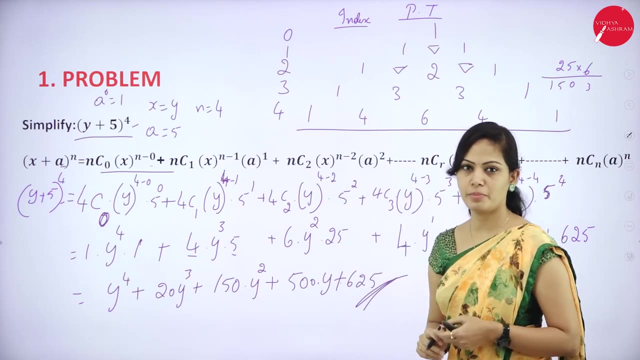 5 terms are there. So this is the final expansion. Very simple concept. Please use this concept called binomial expansion. So this is the expansion formula. Use this expansion formula and Pascal's theorems Easily. you can score 7 marks in binomial. 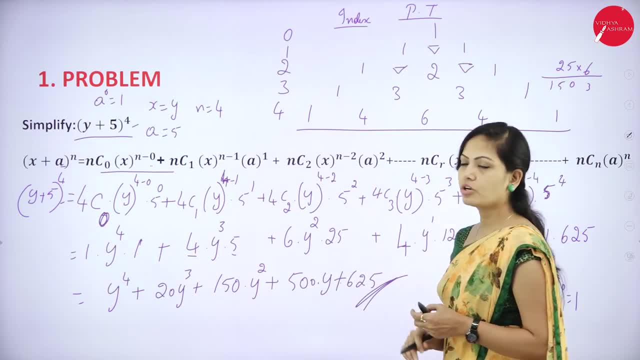 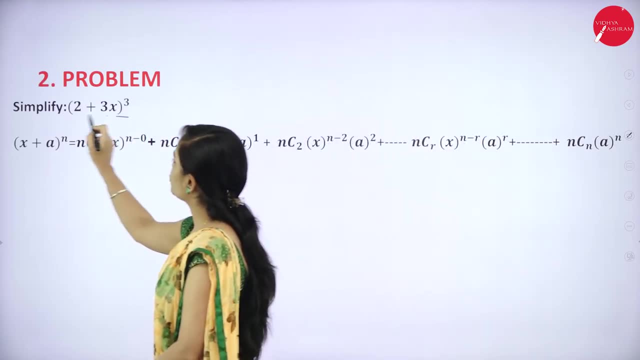 coefficient Clear. So it is very simple concept. Please practice the problem so easily you can understand the logic. And the next problem is second one: 2 plus 3x power 3.. So here n value is equal to 3 and x value is equal to 3.. So this is the final expression. So, this is the final expression. 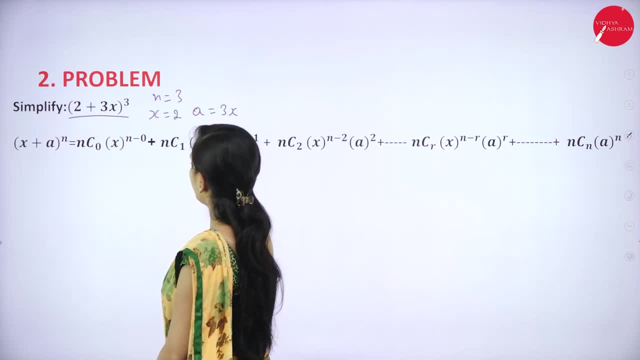 So what you will do is in the next problem. So after 3 sizes only, you will do that again. youngest number of 2 as per 3, then expectation 2 is equal to 2 and the next number, volcano, is equal to 3if it is 3, then nutritional value is 3.. So just remember these 3ибо these. 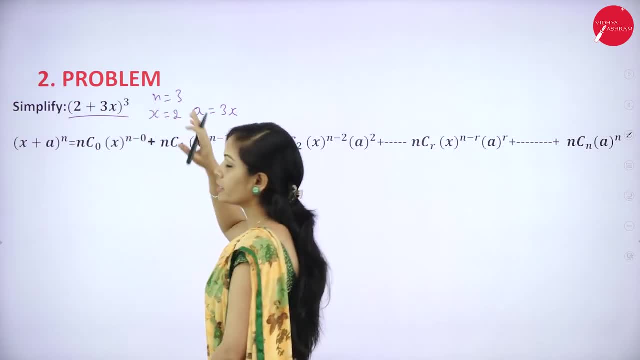 here are the single terms now just doody-boy, right triggering. And the same thing will happen when you do two more and this is equal to 2, and the same thing will happen when 2 is equal to 2.. So we prec Loud: second law has 3 and change it to 2. we don't have the 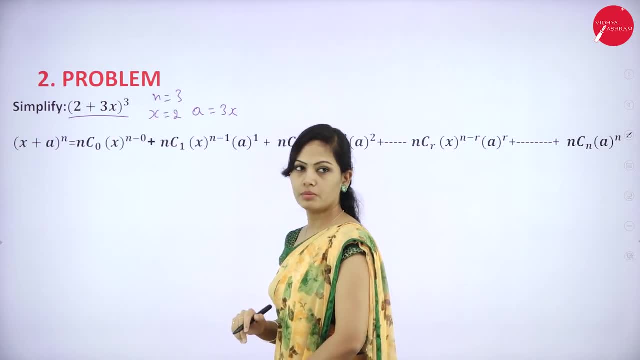 last number to be approximately. We don't have ourselves say, though, that as far to get 3, and instead we have a divide 2 also. so this is for the second kinx, and this is for n and X. So what will happen if, when you have second 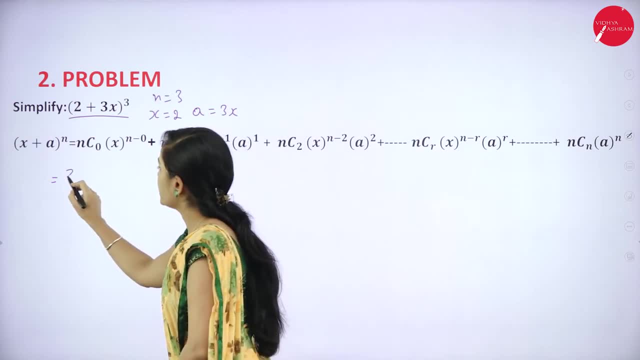 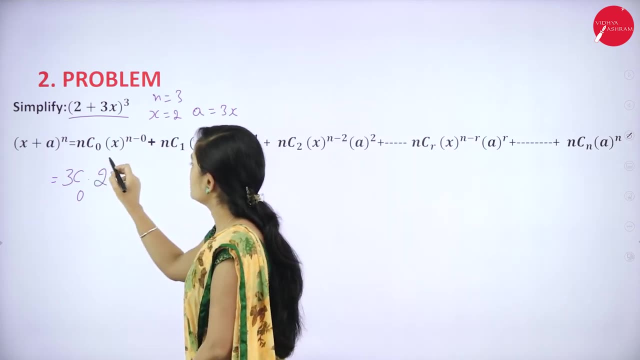 order of n. you trade these 3 for n Because min. Okay, So now who will be our third option? I have 3.. So it is 3C0, and in place of x I have 2.. 2 power n value is 3 minus 0. So the difference. 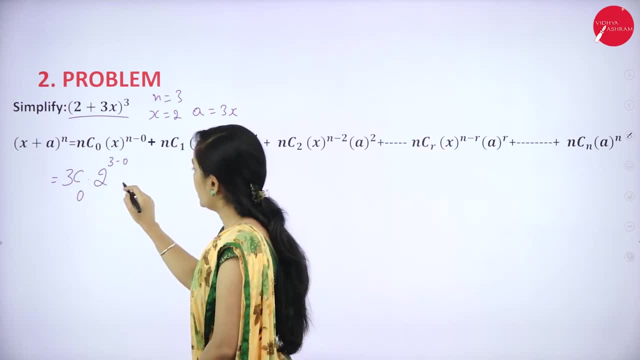 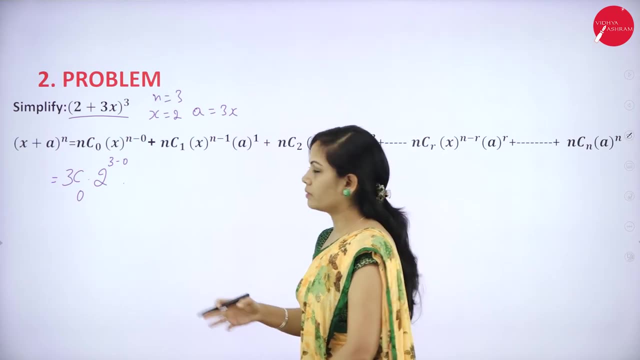 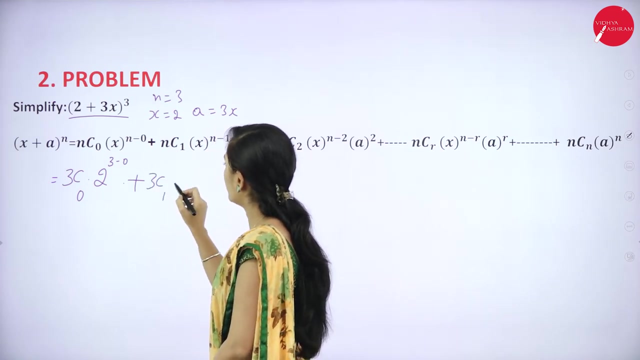 is 3 minus 0.. So 2 power 3 minus 0 into a power 0.. a power 0 means 3x power 0.. 3x power 0 means it is 1.. If you want, you can write 3x power 0 and in next term 3C1 into 2 power 3 minus 1 and. 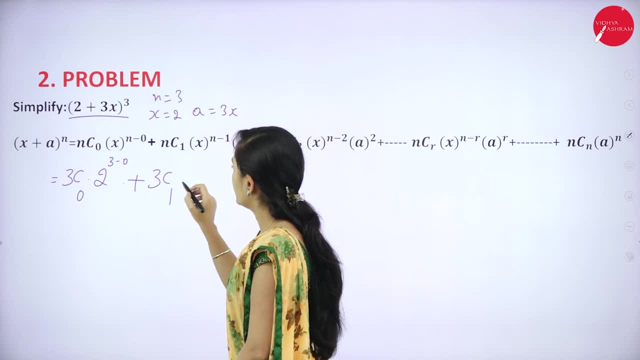 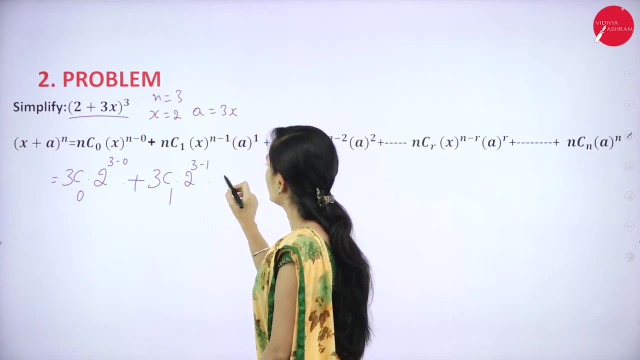 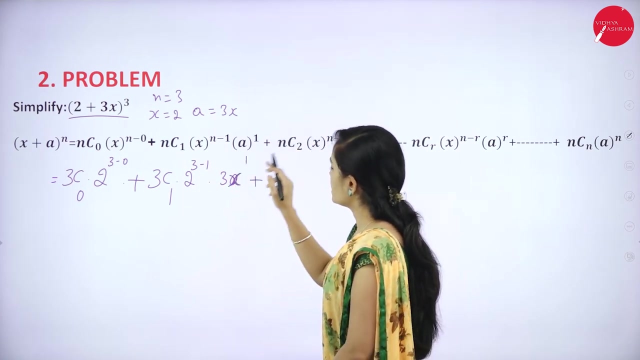 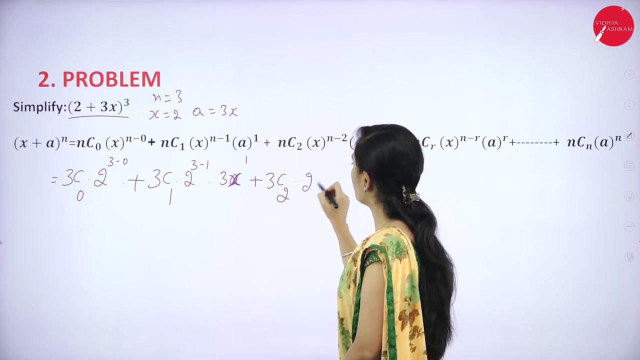 next term. 3C0 changes to 3C1 into 2 power n minus 1, that is 3 minus 1 into a means it is 3x 3x power 1 plus nC2.. This is 3C2 into x power n minus 2.. Here, 2 power 3 minus 2 into 3x power 1.. This is a value 3x. 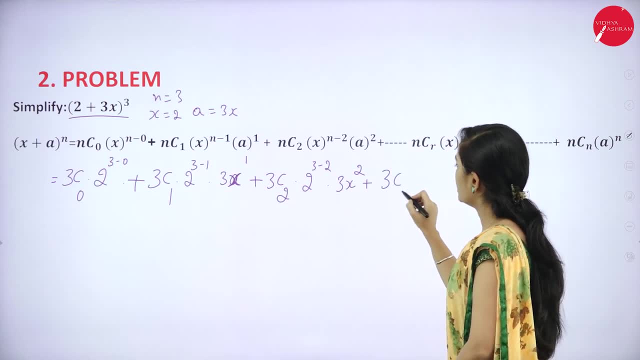 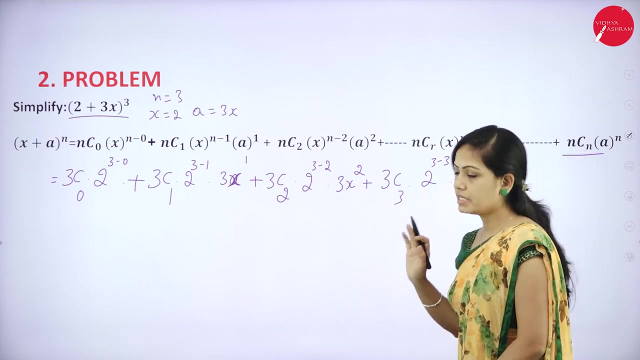 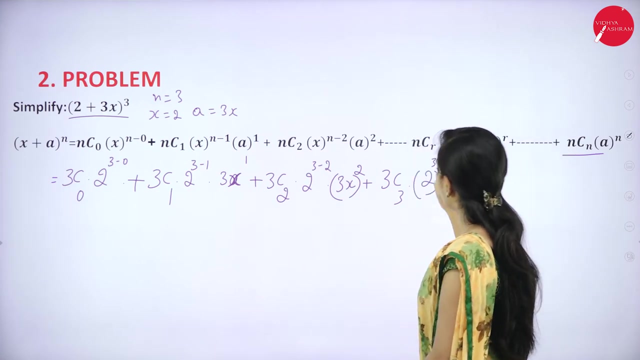 power 2 plus 3C3 up to nCn. you have to expand the expression 3C3 power 2, power 3 minus 3 into 3x power 3.. So here understand this: This is 3x whole power, 2. 3x whole power 3 and 2 power 3 minus 3. 2 whole power. 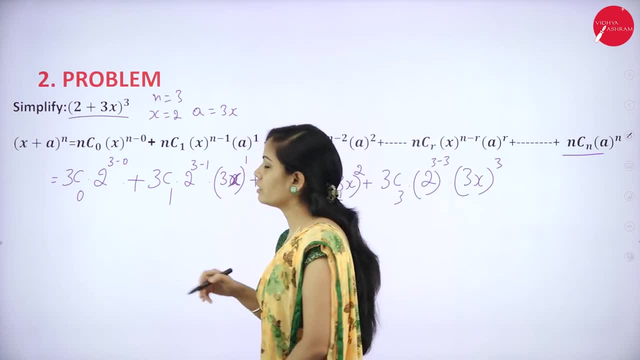 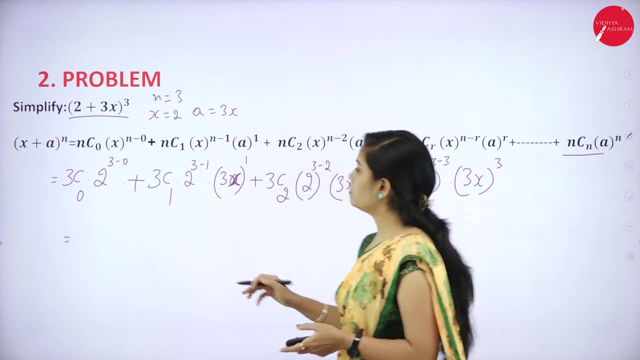 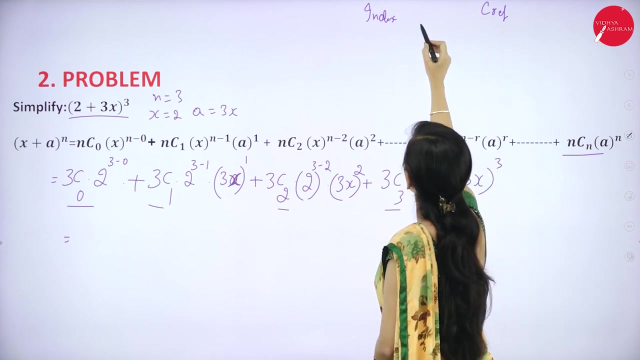 3 minus 2 and 3x whole power 1 and 3x whole power: 0. Please use brackets. and now I will use Pascal's theorem for finding 3C0, 3C1, 3C2, 3C3.. So how to apply Pascal's theorem? Index is 0,. 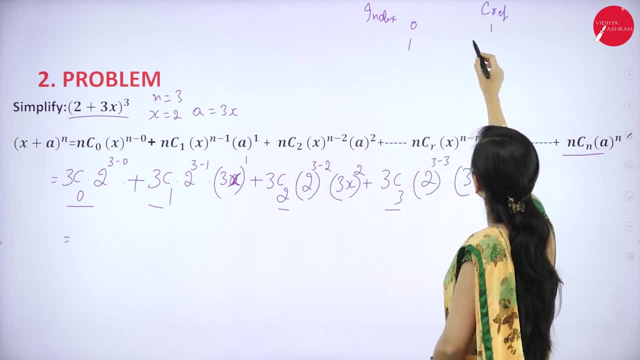 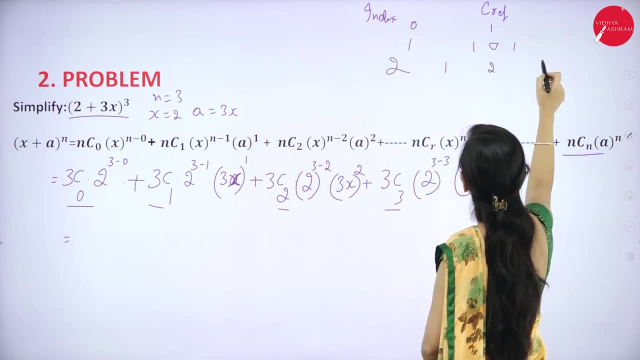 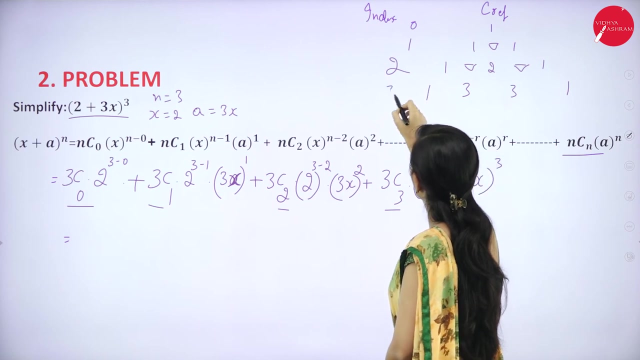 coefficient is 1.. Index is 1, coefficient is 1, 1, 1, 1, 1.. And index is 2.. 1 plus 1 is 2, as it is. I will write 1 and 1 here Again: 2 plus 1 is 3.. 2 plus 1 is 3, as it is 1 and 1.. This is for 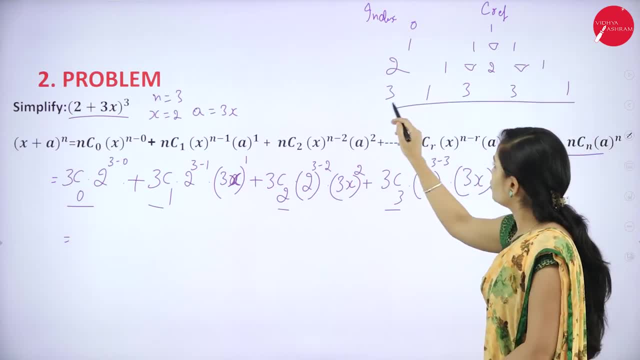 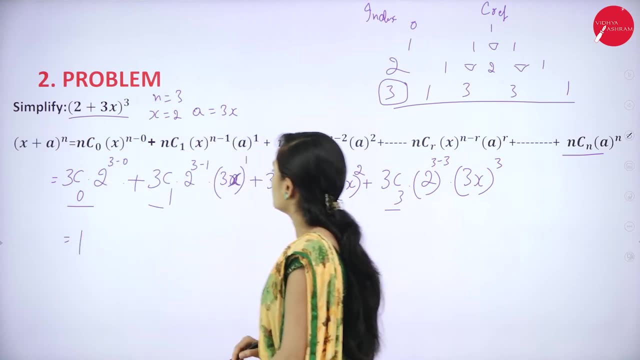 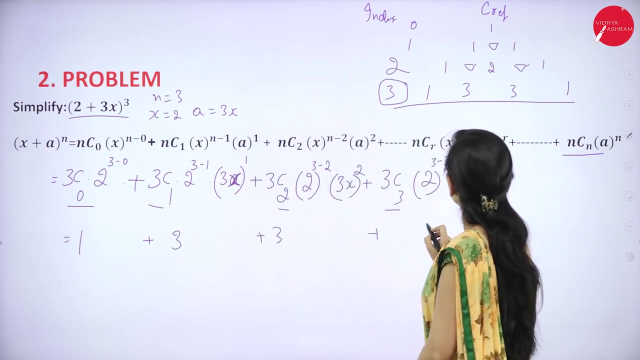 coefficient 3.. So here I will apply these values for index value 3.. 1,, 3,, 3,, 1.. So in place of 3C0 you can put 1.. place of 3c1, which is 3,, 3c2, 3,, 3c3, 1.. So 1,, 3,, 3,, 1.. Now you can simplify this: 2 power. 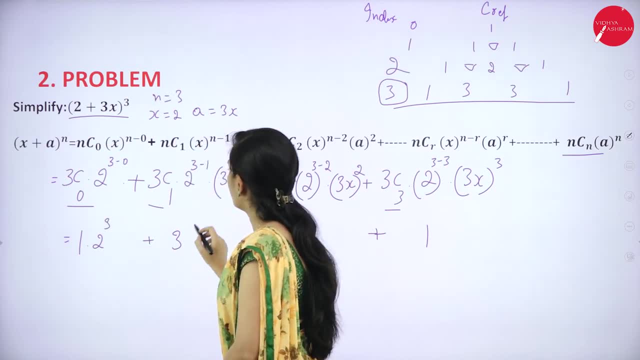 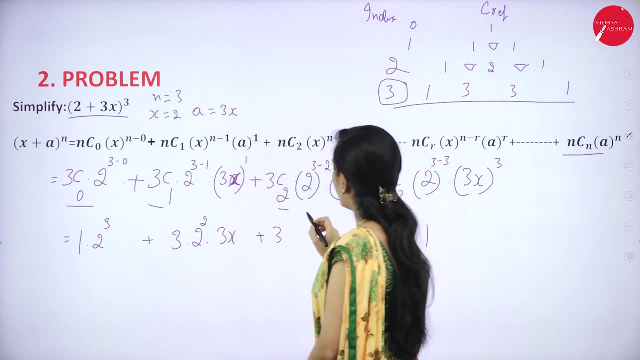 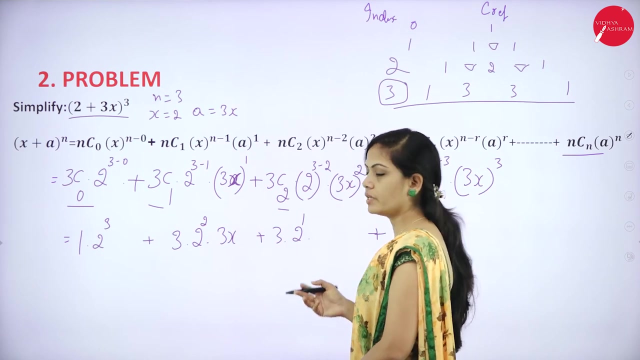 3 minus 0 is 3 and 2 power 3 minus 1 is 2. power 2 into 3x power 1 is 3x and 2 power 3 minus 2 is 1.. 3x power 2, 3x whole power 2, that is 3 into 3 is 9, x into x is x square. 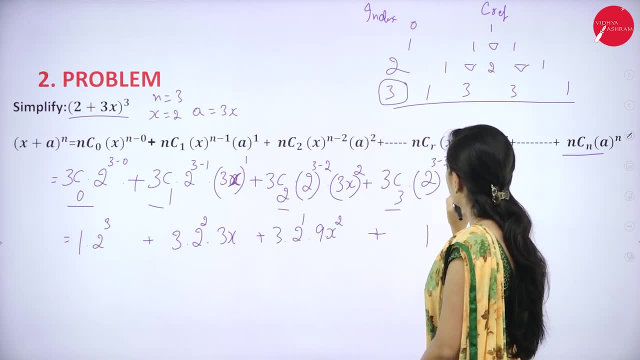 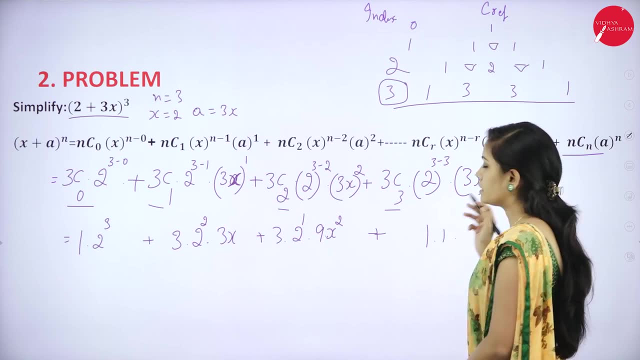 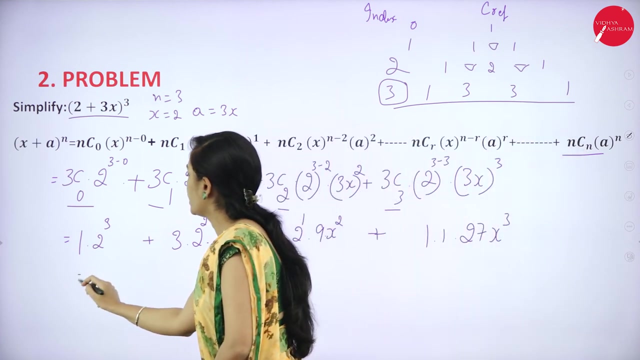 So 9x square. and next is 2 power 3 minus 3, 3 minus 3 is 0.. So 2 power 0 means it is 1.. 3x power 3, so 3 into 3, into 3, 27x cube. Now I will write the final expression: 2 power. 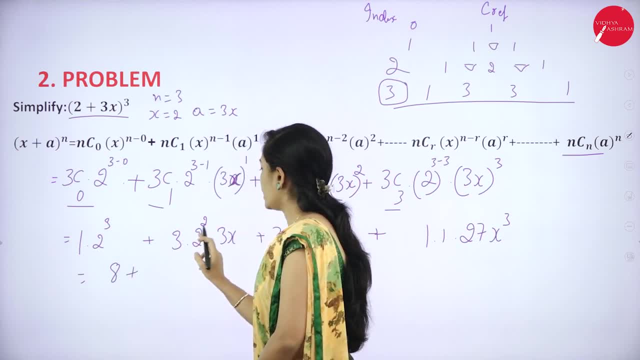 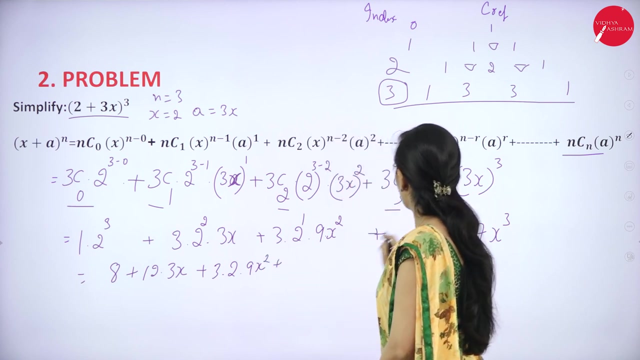 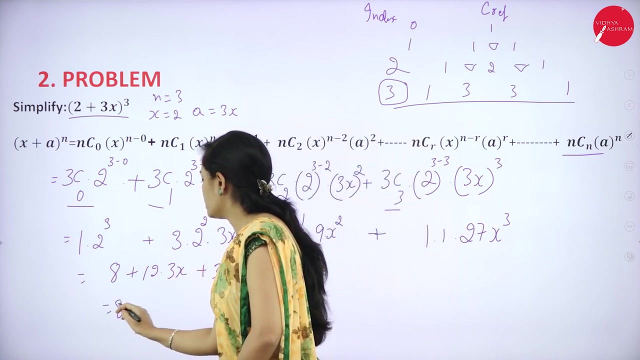 3 is 8 plus 3 into 2. power 2, 2. power 2 means 4, 4, 3 is a 12 into 3x plus 3 into 2. power 1 is 2 into 9x. square plus 1 into 1 is 1, it is 27x cube. Multiply this 8, 36x plus. 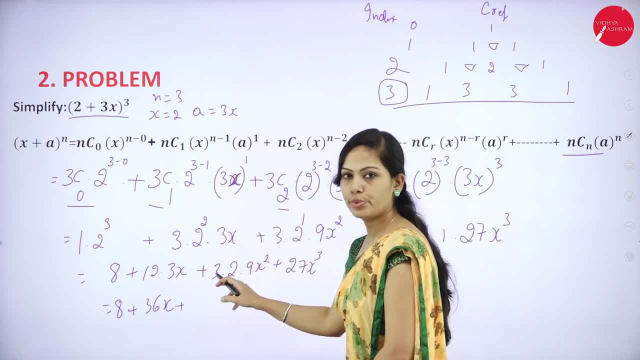 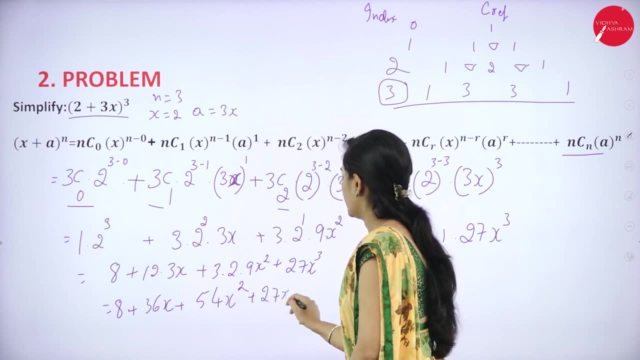 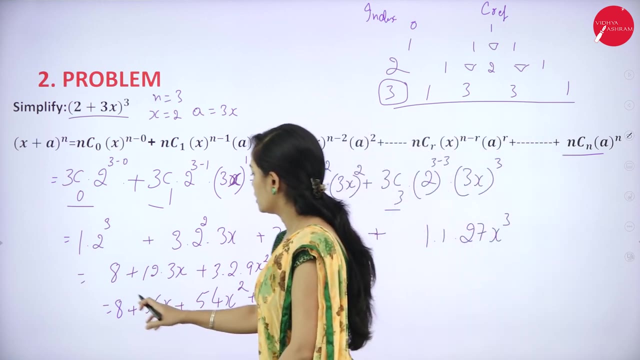 and next term is 9,. 3 is a 27,. 27 into 2 is 54x square plus 27x cube. So this is your final expression. Is there any mistake in calculation? Please find out this: 8 plus 12 into 3, 36, 3 into 2 is 6,. 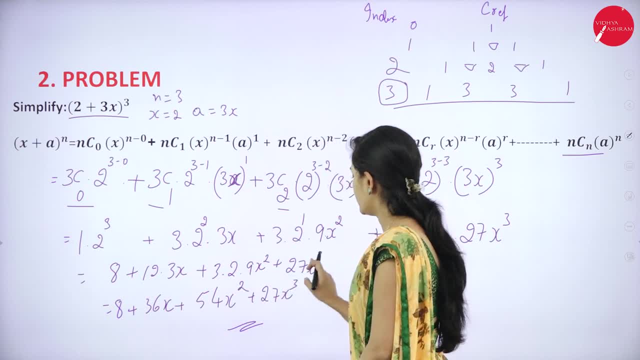 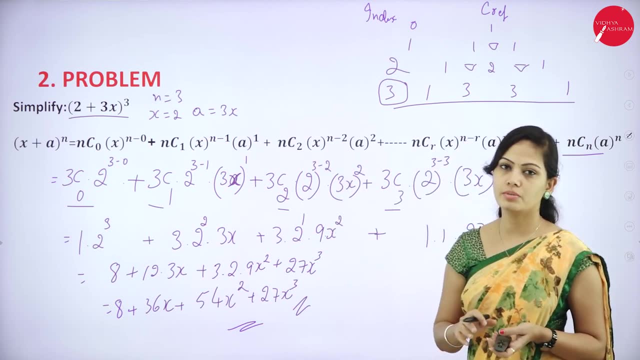 6 into 9,, 54 and 27x cube. So this is the final expression. So here I have used Pascal's theorem and binomial expansion. What is the problem? It is very simple concept. Easily you can score 7 marks in binomial coefficient.